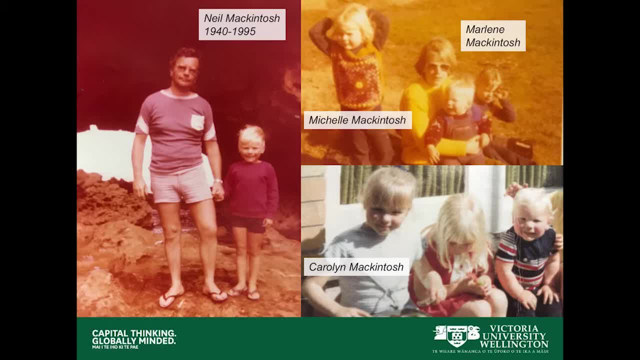 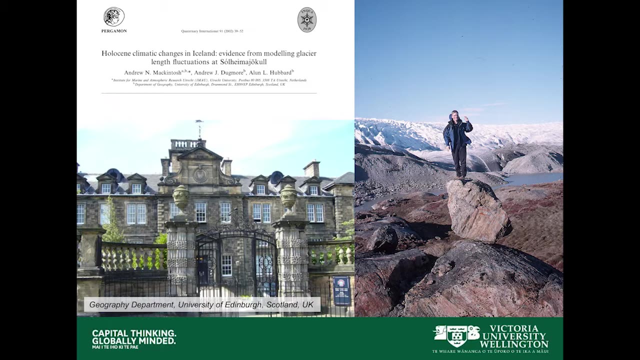 me much direction, So they were not telling me what to do. They just were sort of happy with whatever we did, and that included sort of indulging trips into the mountains and so on when I was a teenager. But I kind of felt like I really got free as a man in my early 20s and went to the UK. 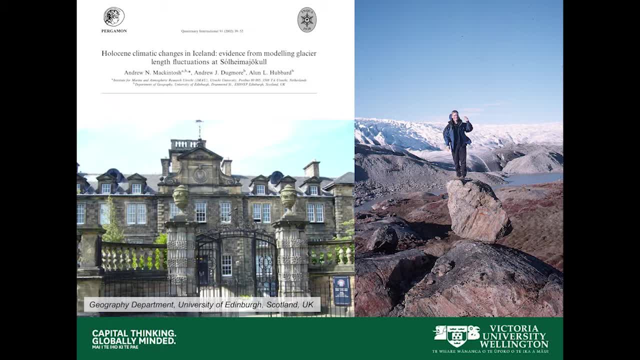 to do a PhD in Edinburgh- and you can see my former department there- and it allowed me to go into the mountains, to go to Iceland, where I worked on a PhD on real glaciers. So Australia, as you probably realise, doesn't have any glacier ice, so here was a chance. 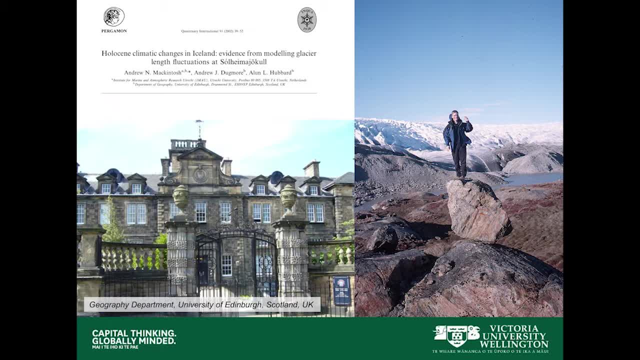 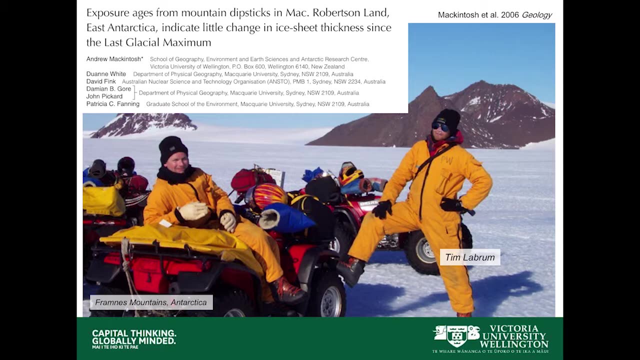 to learn about real glaciers and how they worked and I also sort of learnt some skills in numerical modelling and the kind of computing side of glaciology. when I was there And when I came back I went to Antarctica for the first time with the Australian program. 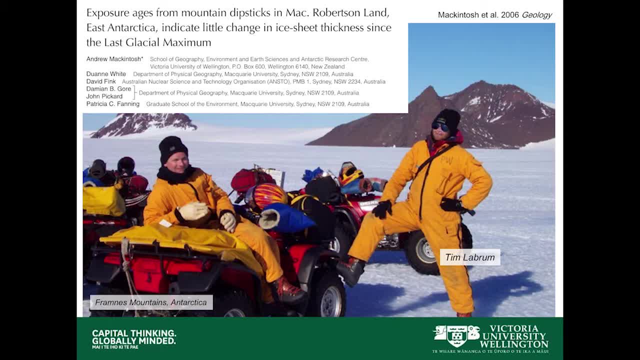 We took a boat to Antarctica. you couldn't really fly down there from Australia very easily. We got stuck in sea ice for six weeks. So during that time I actually signed a letter accepting the position as a lecturer here at Victoria University. That was in 2001.. 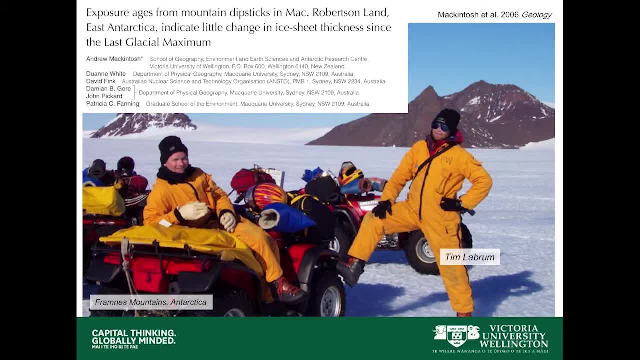 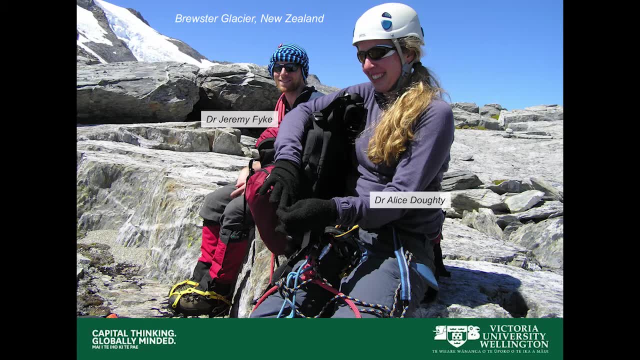 So yeah, this is sort of almost over and into the science. and coming to New Zealand was fantastic. I'd actually never been here before. I did a telephone interview and this was sort of before things like Skype were really popular. I'd never been to New Zealand, but of course New Zealand's a fantastic place. 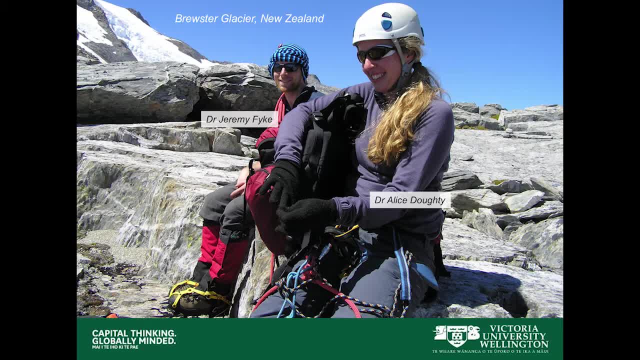 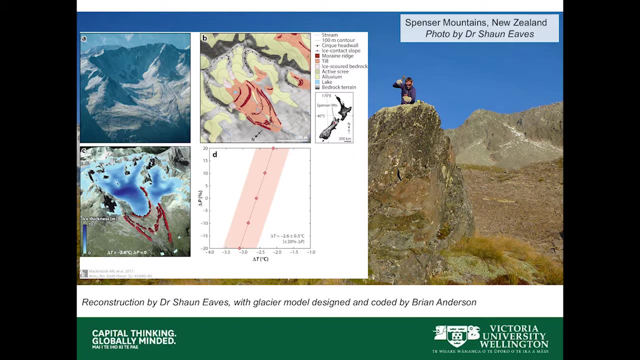 So for the last nearly 20 years I've been enjoying the mountain scenery in New Zealand, working on real glaciers, and I've been privileged to have a group of fantastic doctoral students in particular, So you can see two of them here Now. we sort of started something which I think many people are doing these days, and 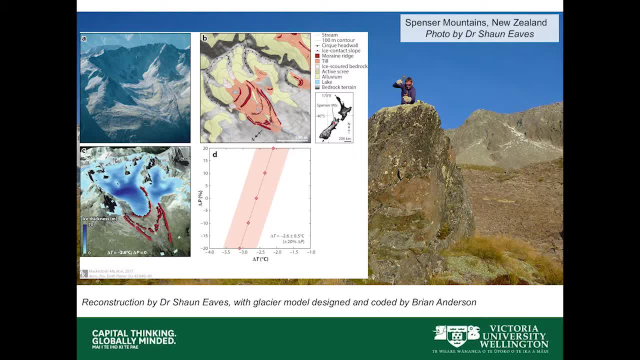 that's bringing together understanding of landscapes- So you can see a beautiful mountain landscape here in the Southern Alps- dating landscapes using quantitative methods- and I'll talk about that a bit more later- and then bringing that together with computer models to understand climate. 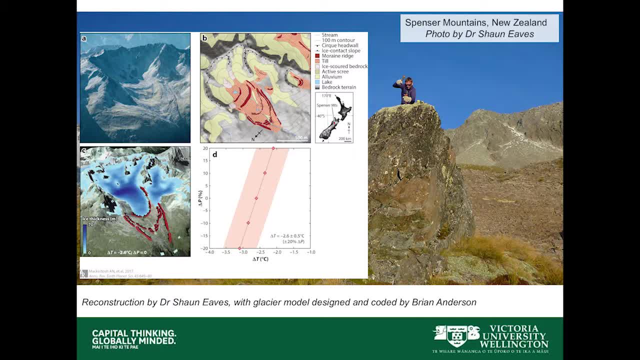 So here's my first bit of science. You can see a mountain landscape in panel A in the Southern Alps, the mapping of that in panel B. Panel C is a numerical reconstruction of the glacier that once sat in that basin, and panel D is a reconstruction of the climate from the climate. 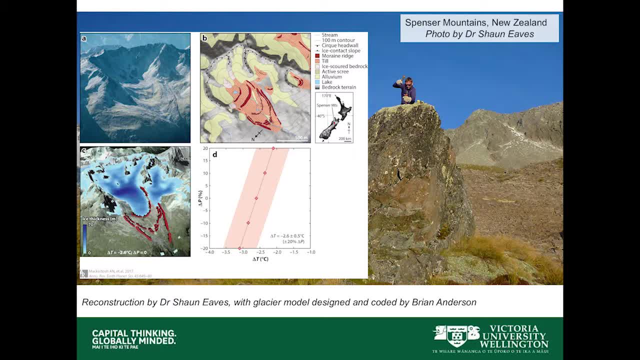 So you can see a beautiful mountain landscape in panel A in the Southern Alps, the mapping of that in panel B, Panel C, the mapping of that in panel B, the mapping of dynamics in the right of like the beneficial, and you can actually see the hoch зв. the knowledge of theAST can be reading. 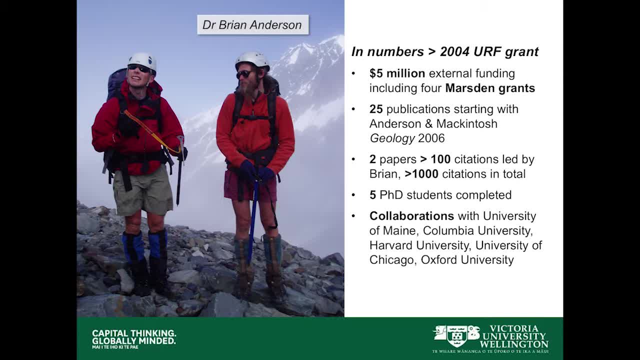 comfortably. You can see the destroying grip became clear. three publications to my name. the university invested a hundred thousand dollars in me in the URF grant which I used to employ- Brian Anderson, who's somewhere here in the audience, and since then we've brought in five million dollars of funding. four Marsden grants, 25 papers. 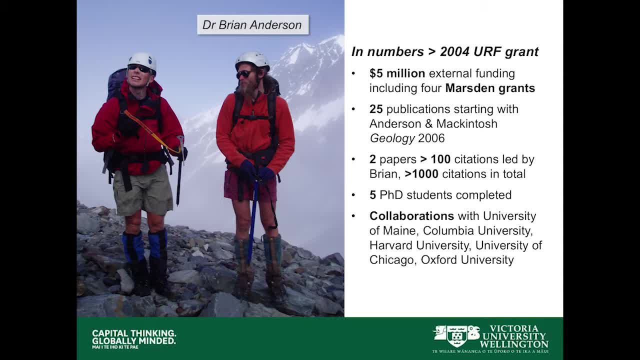 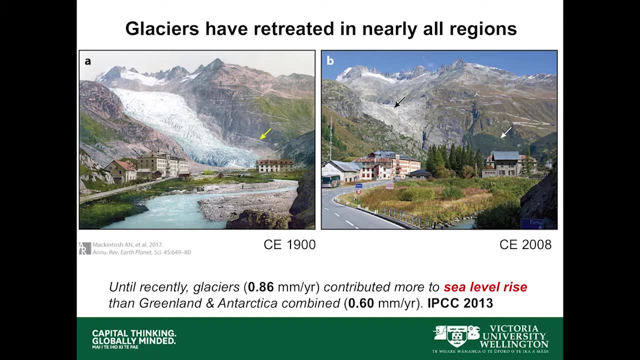 five PhD students co-supervised. anyway, I just wanted to say thank you, invest in your young staff because you know that it can really pay off. anyway, much of the work that I'll talk about now has been collaborative with Brian anyway, so that's my little introduction. I think I've 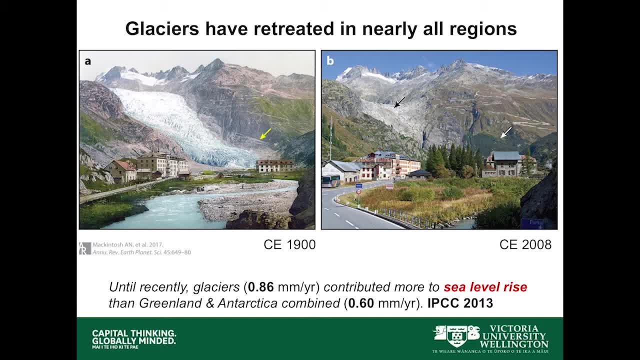 gotten over my moment, and so let's talk about glaciers to begin with. right, they've retreated in nearly all regions on earth. this is a from a paper I wrote recently. it's a European glacier, the Rhone Glacier in Switzerland. you can see how it looked in 1900, and then 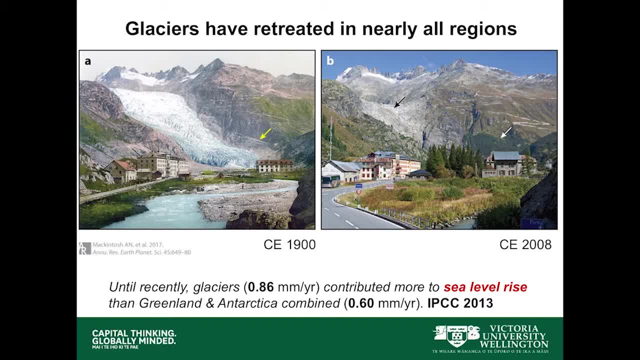 it looked in 2008. it's even smaller now. this is something we've seen, no matter which mountain range you go to: a dramatic retreat of mountain glaciers, and until recently, glaciers have contributed more to sea level rise than ice sheets. both ice sheets combined, we've got two big ice. 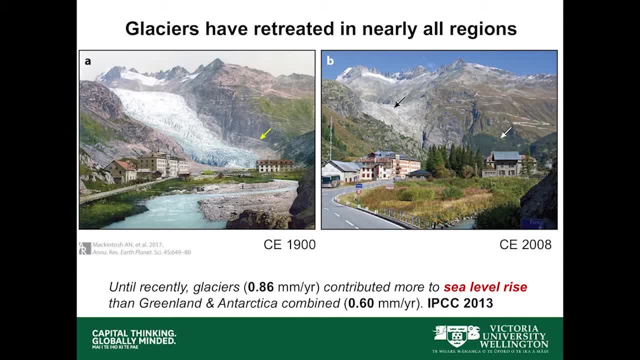 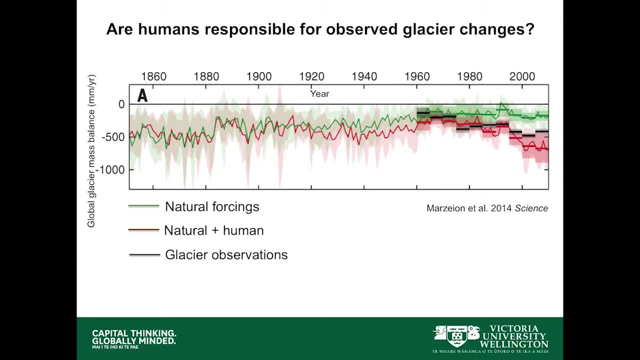 sheets in Greenland and Antarctica, and the little glaciers were almost putting as much water into the ocean. that's just now changed, but they'll still continue to add water to the ocean for a long time. this is another one of my sort of more complicated science slides- not just photos and so on, but it's. 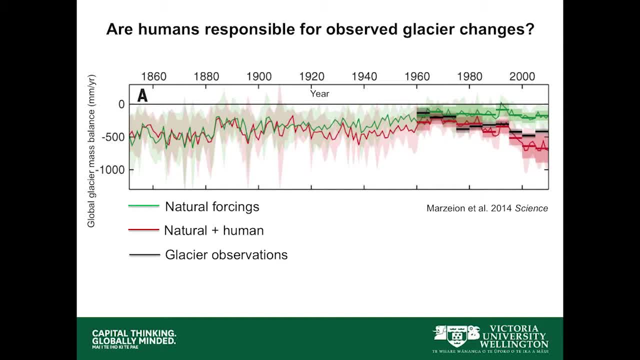 it's worth. it's worth looking at because the critical question is: have the have retreating glaciers? has that retreat been caused by humans? right, many people ask this- it's a common question, you see- in the media or by climate change skeptics, and the answer lies here in this graph, and 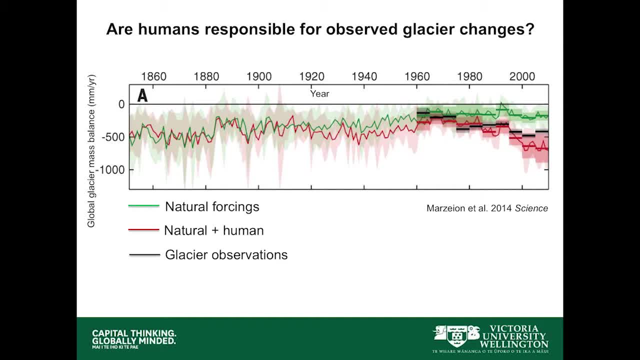 what you can see here are a few different simulations with a climate model that are used to model right on the y-axis. you can see negative 500, negative a thousand. the more negative is the, the worse it is for a glacier. and then time on the y, on the x-axis, from 1860 to 2000.. 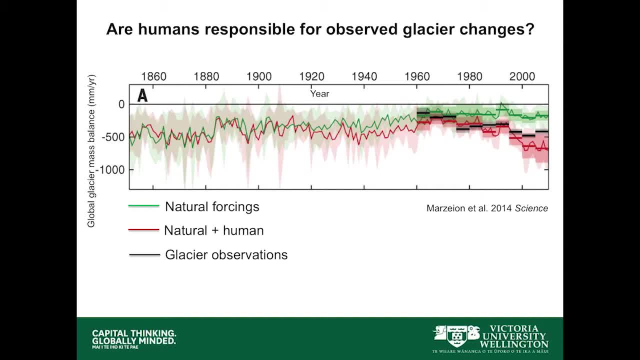 the green line represents a simulation of glaciers in a world that is just including natural forcing of climate, so volcanic eruptions, solar variability and all the complexity of atmospheric circulation that occurs on earth. the red line is what happens to the glaciers if you then add human induced climate change, anthropogenic forcing and the black 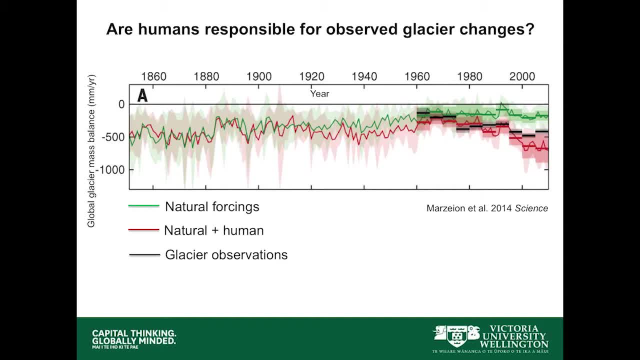 lines are observations, and what you should be able to see there is that the black lines look much more like the red lines and not at all like the green lines, but only after about sort of 1980 or so and after about 1990. in fact, two-thirds of the forcing of glaciers has been by humans and it's 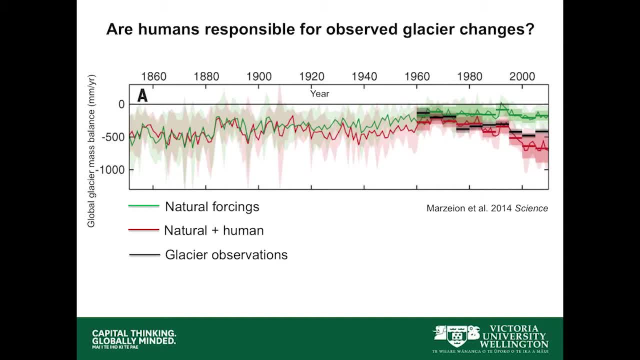 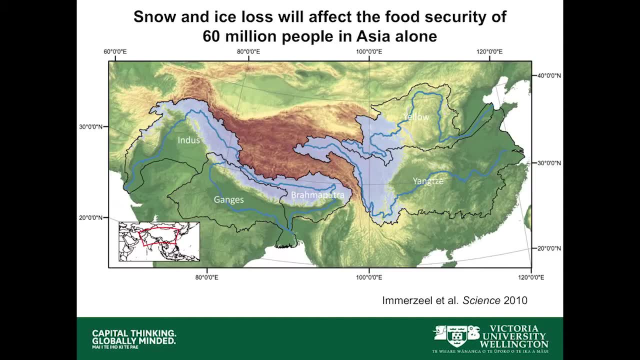 getting more and more every year. so to answer that question, are humans responsible? yes, but only for the last few decades. before that was natural variability, so it's never just black and white, right. so some combination. why is this important? um, of course, new zealand glaciers are important to us, but uh, if you want. 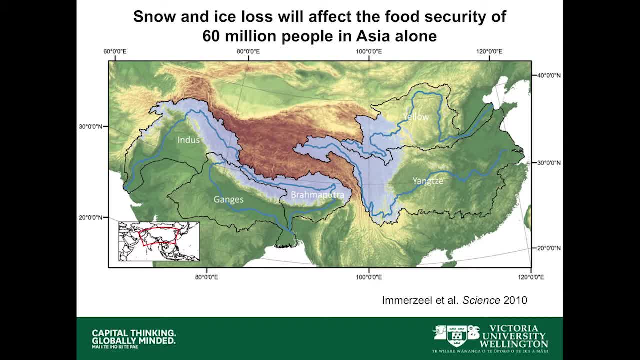 to really know why this is important. apart from sea level rise, the effect of changing glaciers on water supplies will be profound. now there are billions of people who live in central asia, but the ones who are directly affected by changing snow and ice melt in the major river basins of central asia, like the ganges, india. 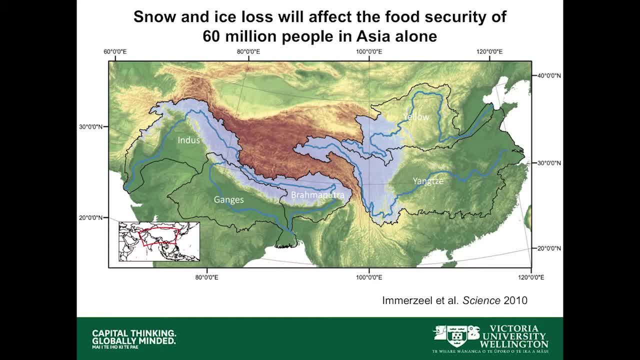 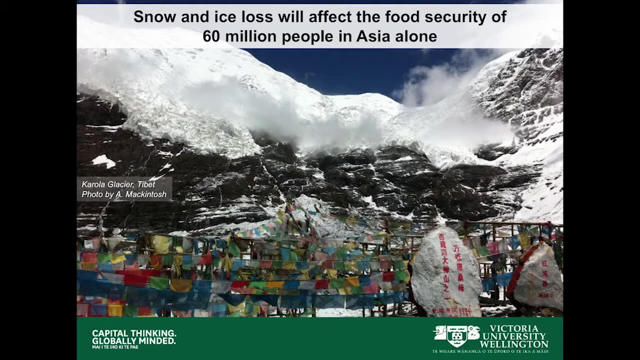 is brahmaputra and yangtze. 60 million people alone are going to be affected by changing snow and ice in the near future. the blue just represents the area above about 2 000 meters of sea level. i've never worked in this area, but i've spent a bit of time there as a tourist, and you can. 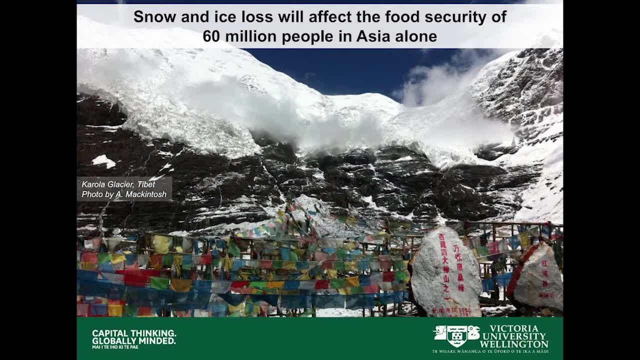 see what it looks like up high in the himalayas, and this is a photo from tibet. and so there's this, these sort of frozen water resources sitting on tops of the mountains. in fact, there's more. there's more ice in uh central asia than there is in central asia, so there's more ice in central asia. 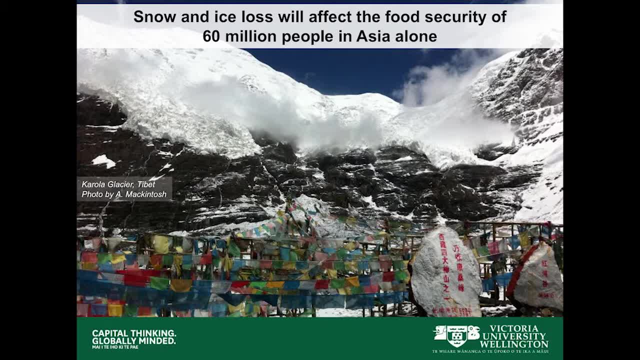 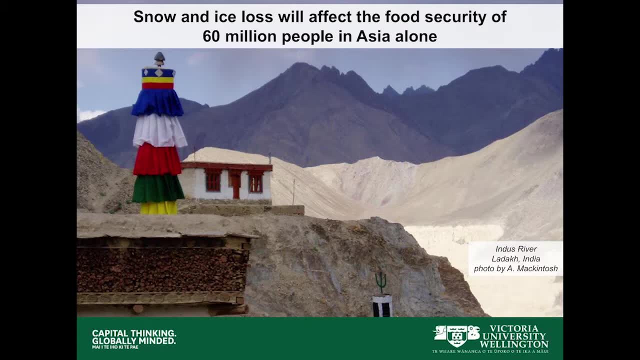 than anywhere else in the world, apart from the polar regions of greenland and antarctica. but then in some drainage basins like the indus, it's so dry that you can imagine that melting snow and ice is the only source of water, right? so if it's gone, then the people just won't be able to irrigate. 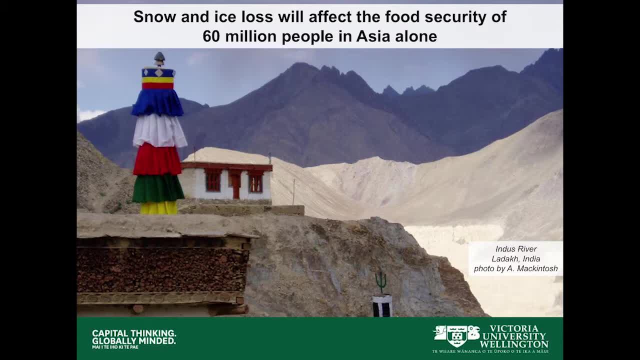 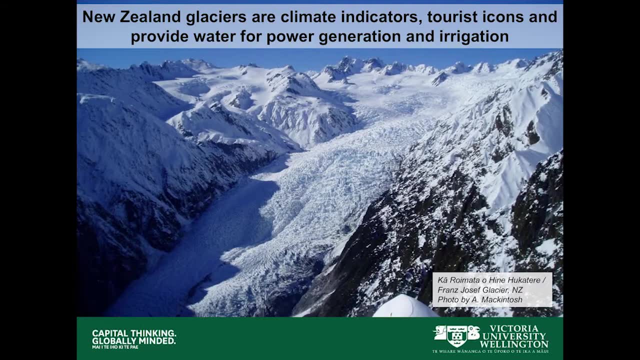 their crops or run their hydropower or anything right. so in some parts of the world snow and ice is just a critical water resource. in new zealand it's also an important water resource, but it's not critical. it rains a lot here, so in the southern alps the combination of rain, seasonal snow melt and melting glacier ice- all 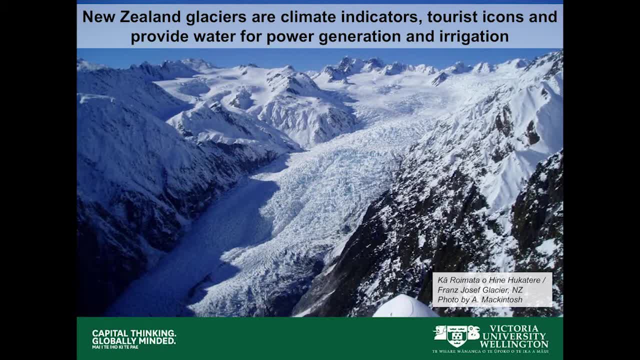 contribute to our water resources. we've recently been funded by the deep south national science challenge to do some predict projections of of snow and ice to try to help answer the question of what might happen to glaciers and snow in the future. i'll show you some of these simulations in. 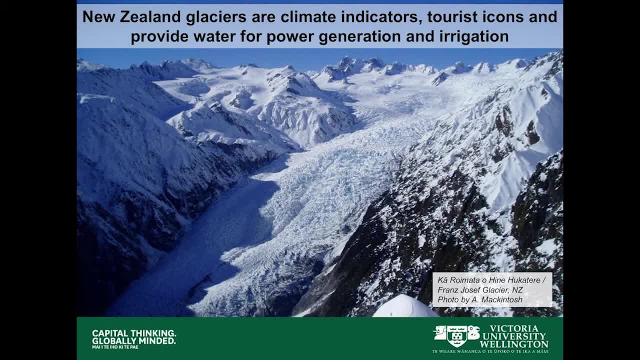 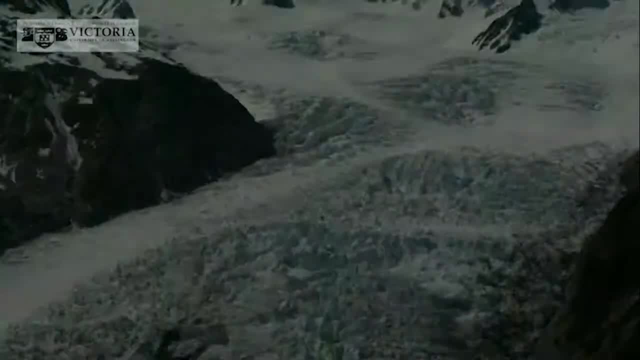 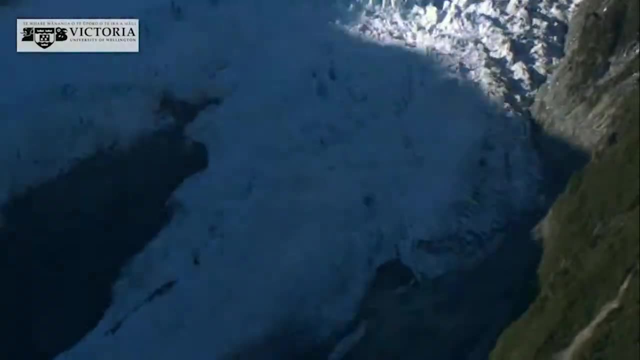 a minute. so let's start off by showing you one of these wonderful time-lapse videos by brian of france, joseph glacier, um the maori name karomaita or hinohukatera- the tears of hinohukatera. so it's a really wonderful um story about uh hina, who was walking in the mountains. 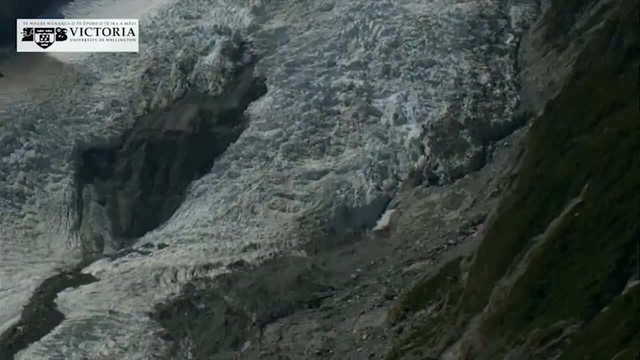 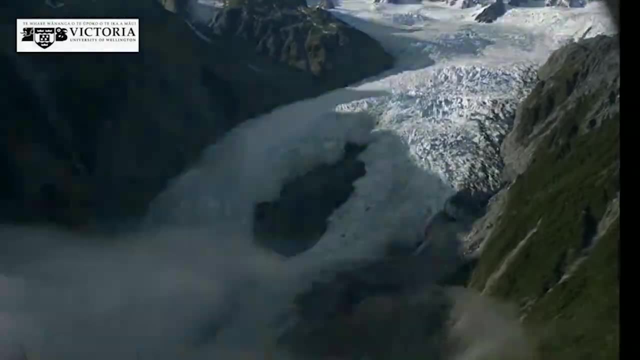 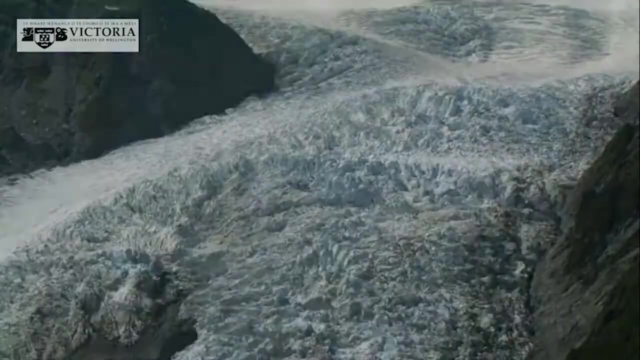 with her partner tawe, and he fell to his death and hina cried and her tears became frozen and became the france joseph glacier. see it in in this um, in this movie, right? so that's a wonderful illustration of how new zealand glaciers move. what they're doing is transferring mass from high in the mountains where there's 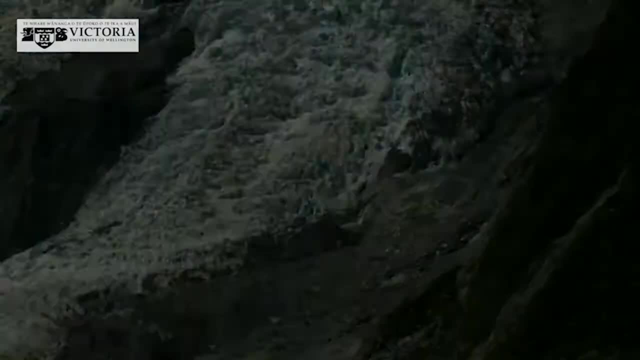 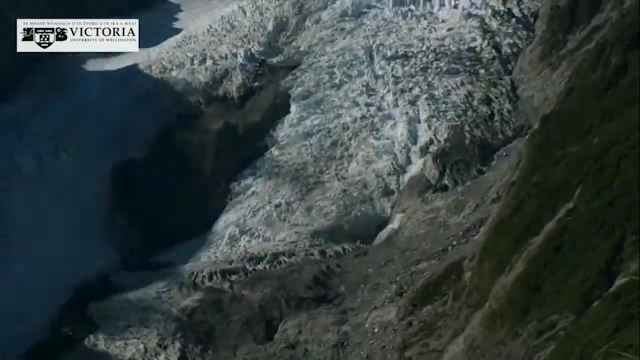 more than 10 meters of snowfall a year. they're traveling downstream here at about a kilometer per year and they melt by about 20 meters a year vertically at their terminus, which, mind you, is the most melt ever observed by any glaciologist. 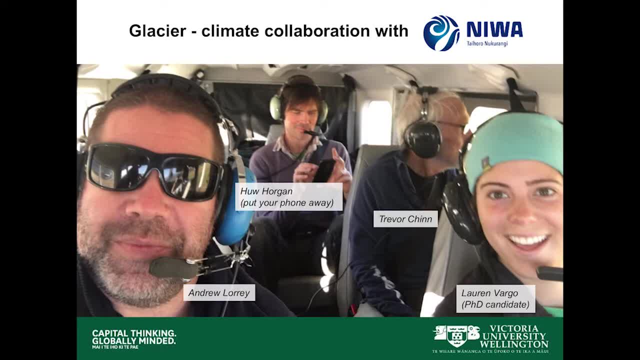 on earth, measured by brian. so for quite a while now we've been studying glaciers and we do this at the moment almost exclusively in collaboration with with niwa, and you can see this photos from a end of summer snow line flight. so once a year neewa fly around the southern alps. 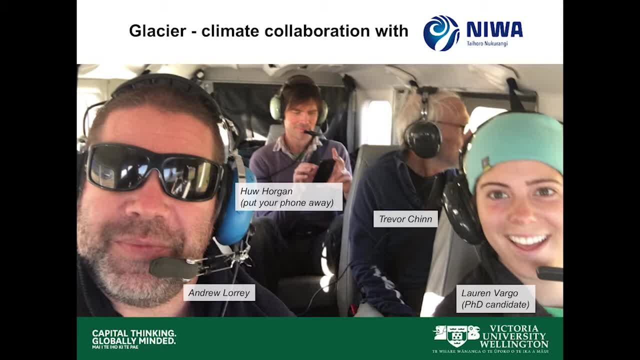 our scientists join this trip. you can see hugh horgan, who's from the antarctic research center, lauren vargo, one of our phd students, and andrew lorry, who leads this, this neewa program, and takes photos of glaciers when they're sort of. 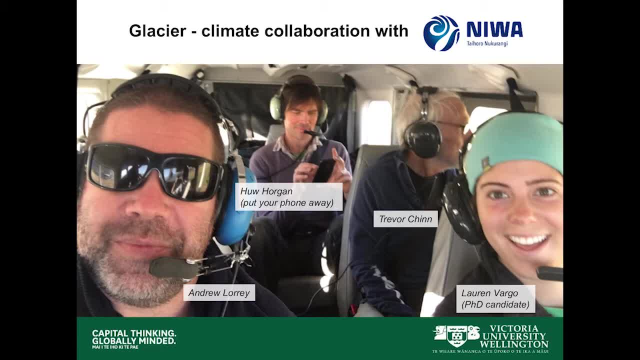 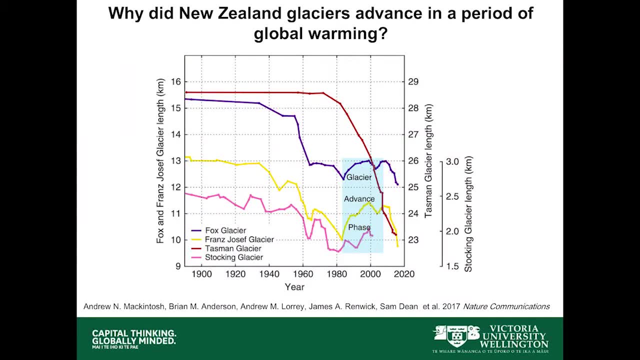 at their worst after they've melted through the summer, and we get a sense of what they're doing with climate from that. i'll show you some pictures in a moment. and um, using this sort of combination of things. i've been talking about direct observations of glaciers and numerical models. 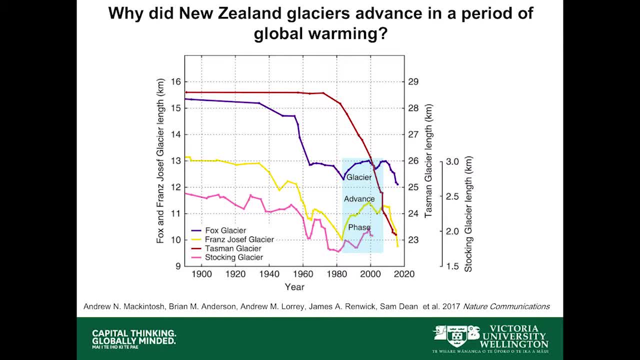 of glaciers- uh photo archives from from these neewa flights. we can sort of put all this together and answer some pretty fundamental questions about glaciers and why they're changing and what's responsible. and one of the one particular problem that really struck me when i first arrived here was trying to understand this rather unusual behavior of 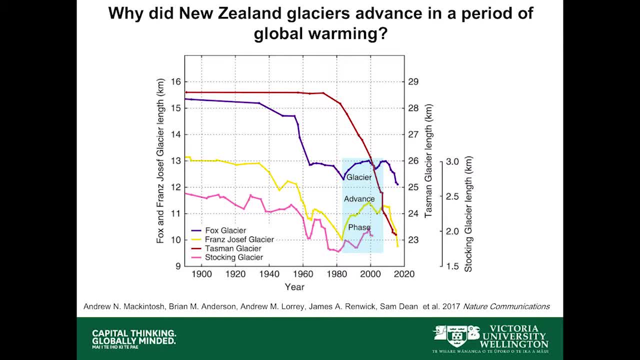 certain glaciers in new zealand, in particular france joseph and fox glacier, advanced through the 1980s and 1990s. france joseph began to advance in about 1982- 83 and continued until about 2000, and during that time it regained about a third of the total length that it lost during the 20th. 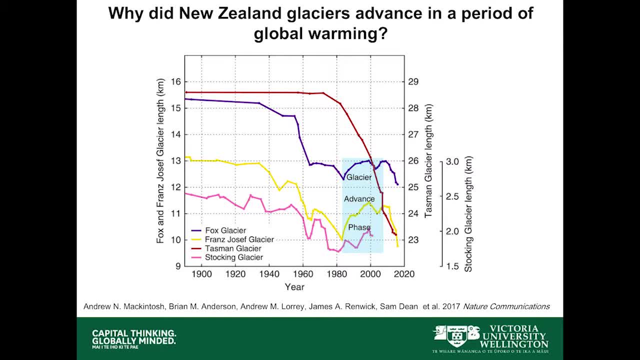 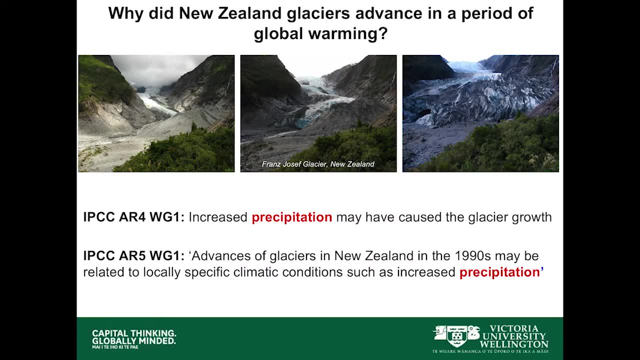 century like remarkable and nobody understood it. what could have caused this? this um, this feature- so it's what i call here- a glacier advanced phase, yep and uh, sort of what it looks like. this is. to be honest, this is a little bit of trickery. um, i've swapped the photos around so it looks like. 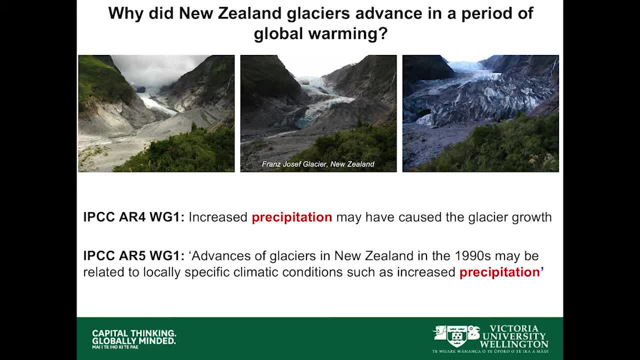 an advancing glacier, but um, but you can sort of see the scale of terminus fluctuations that are possible in these glaciers. that's that flow so fast that brings so much mass down the hill. they can really react very, very quickly. and here you can see a couple of quotes from the last 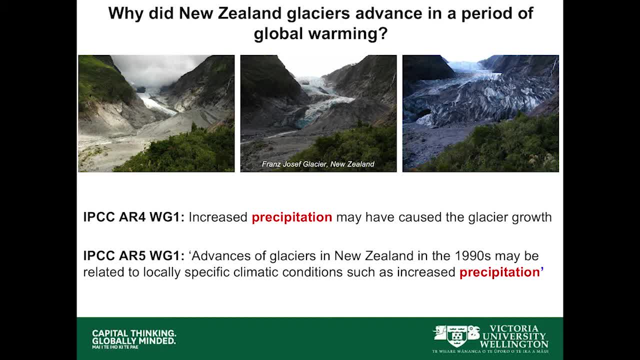 two ipcc reports about why this probably happened. increased precipitation may have caused the glacier growth. and again in the second one, and this sort of makes sense right: in a warmer climate one might imagine there might be more precipitation. there's a physical relationship between air temperature and how much moisture can be held in the atmosphere, so this seems. 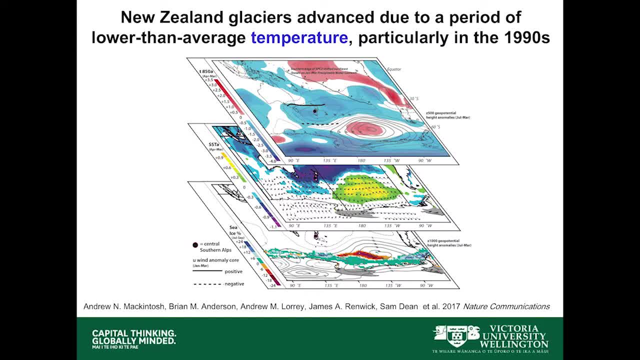 logical, but there's no evidence for it, no actual support. it's just a hypothesis and um, we did some very careful work using glacier models and climate models and climate reanalysis products. again, this is the sort of sciencey bit and this is a three layer plot of the atmosphere. the lower two plots: 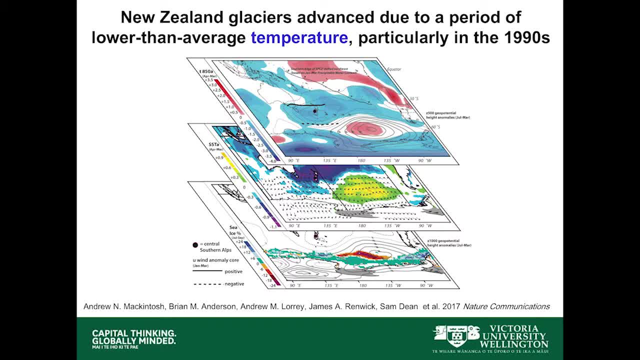 show what's going on at ground level and this is up high in the atmosphere, at about the height of mountains. the blue represents pressure, so blue is low pressure here over new zealand, high pressure waters around new zealand, a high pressure over antarctica and this is changing sea ice, so less. 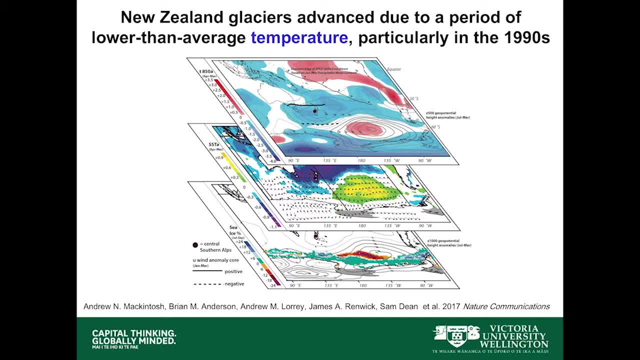 sea ice down in here in antarctica- i'll talk about this in a minute- and a little bit more to the south of new zealand, sort of in the catchment for our weather in the 1990s these conditions dominated and they were an anomaly right. and if you look at the long-term mean temperature change for the 20th. 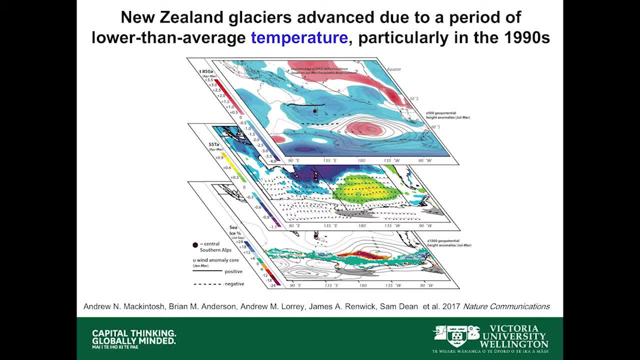 century it's just getting warmer and warmer, but in the 1990s, and so there was a little bit of a blip, but particularly after the pinnatubo eruption in uh in 91, a bunch of el nino events that caused this atmospheric circulation anomaly, that caused it to get colder in new zealand temporarily, and 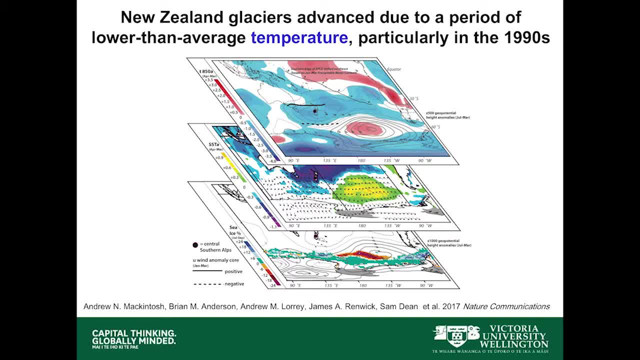 because our glaciers, or at least some of them, are so dynamic and fast flowing, they were able to respond to this short-term cooling and advance right, so that the ipcc statements about increased precipitation are incorrect and it was due to temporary reduced temperature that caused glaciers to advance. this is a very interesting event that i think we can all talk about, and 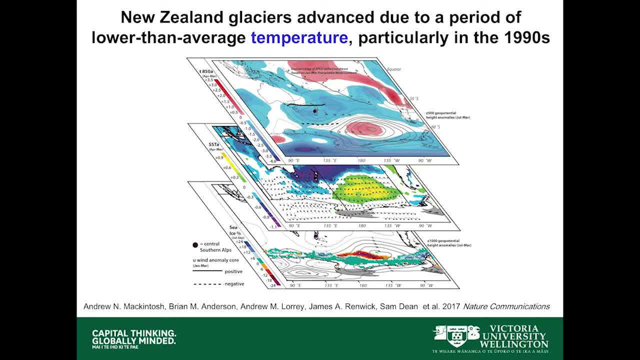 important to know this stuff because, um, now, when a climate change skeptic asks a question, you know why did this happen? glaciers are actually advancing- they're not anymore, by the way- but if I ask that question, there's a very straightforward scientific explanation for it, based on sort of rigorous understanding of 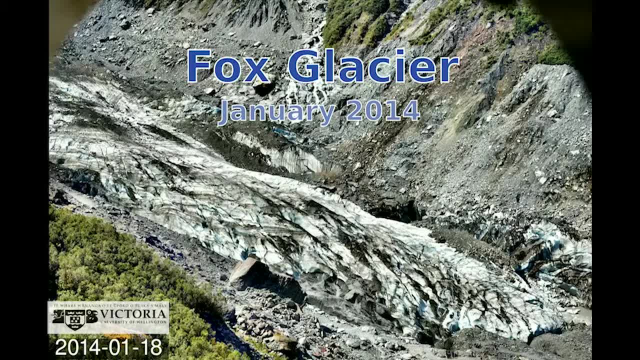 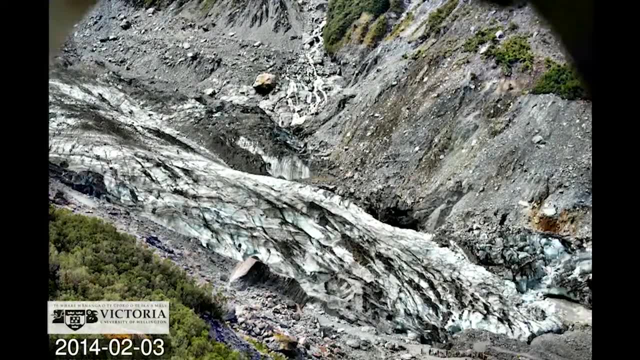 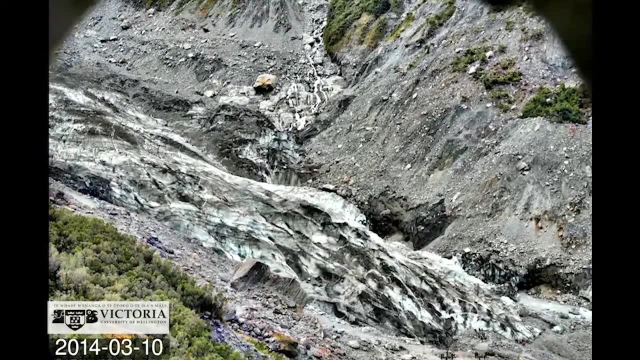 glaciers and climate. right, it's not all good news. so after about 2011, it's been getting warmer in in New Zealand, and this is Fox glacier- another video by Brian- and the first thing you'll notice is the hillsides falling down. right, it's time-lapse video and you can see the hill moving down. it's it's doing that. 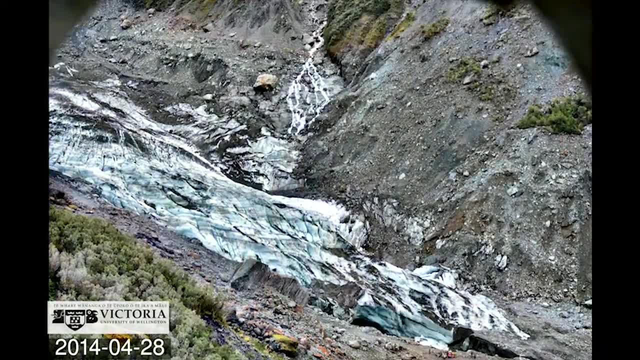 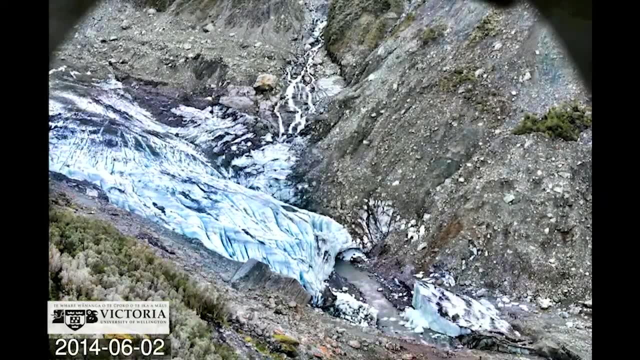 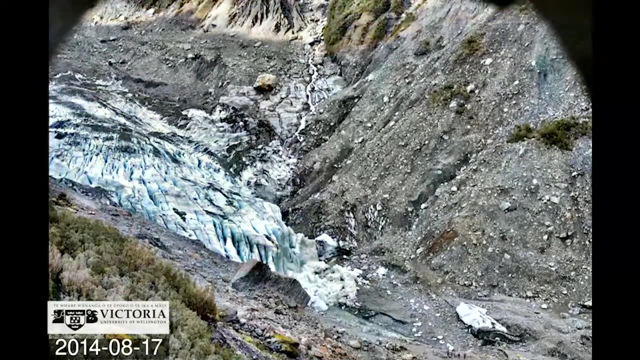 because the glacier is starting to retreat. it's debauchery seeing the slope and very soon what you'll see is the end of walk-on guiding. that was possible at Fox glacier, so about now the glacier falls to pieces and it's no longer possible to walk on to Fox glacier. 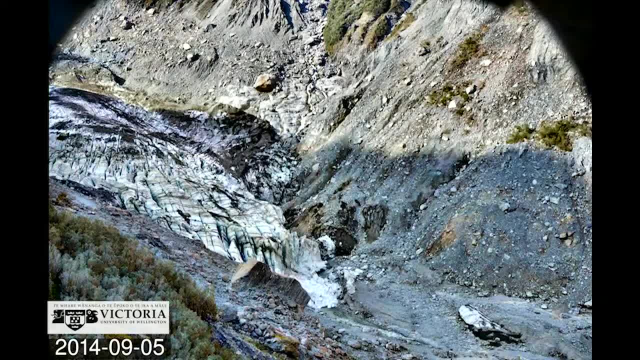 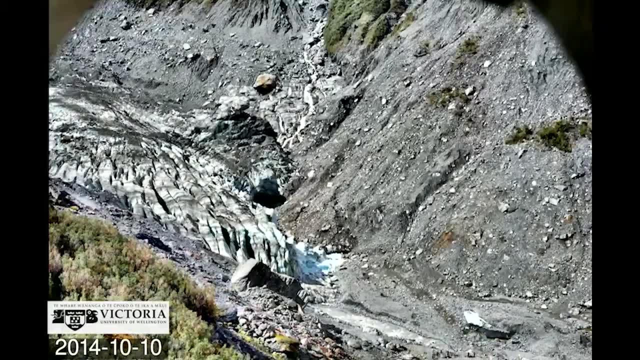 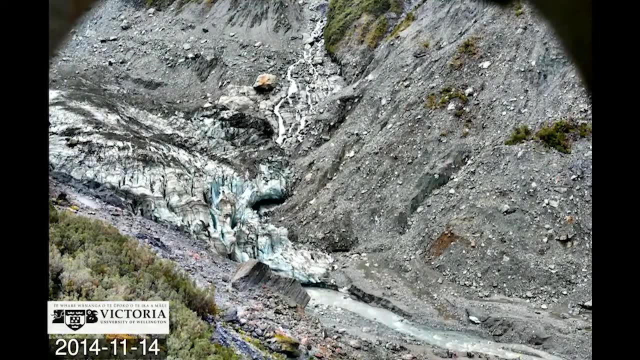 so, somewhat ironically, the only way to go walking on there these days is to take a helicopter, which, of course, burns more fossil fuels, which is contributing to the warming that is causing the glacier to retreat. so, since 2011, it's gotten warmer at Fox glacier. it only takes a few years for the ice to respond. 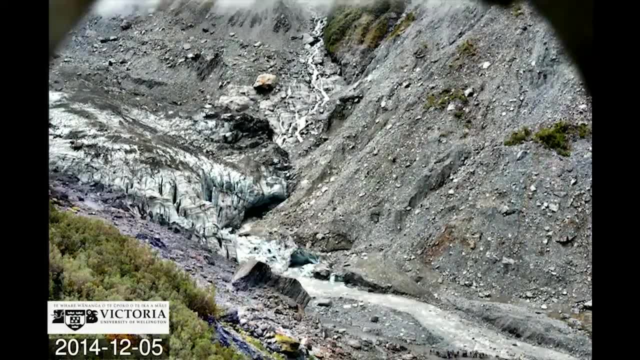 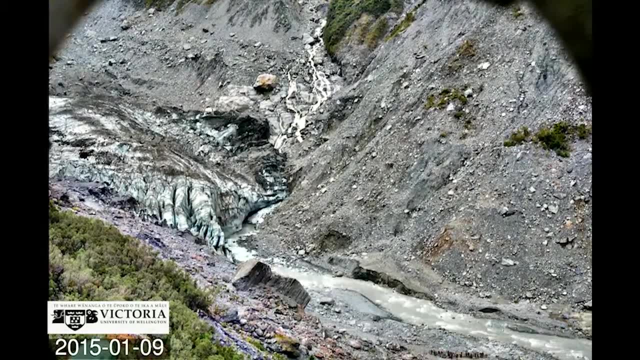 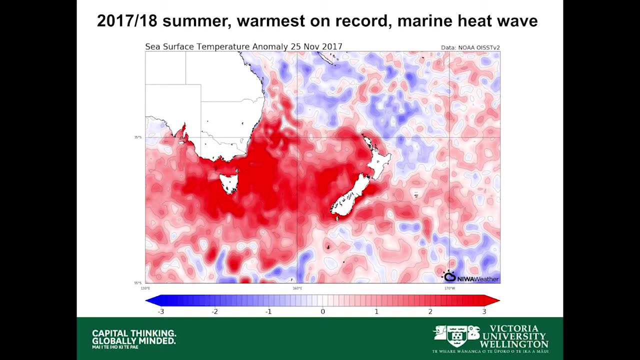 and so by 2014, within six months, you saw about a kilometer of retreat of the glacier. that put an end to the guiding business. it's not good news. in 2017 and 18, we had the warmest summer ever recorded in in New Zealand. I. 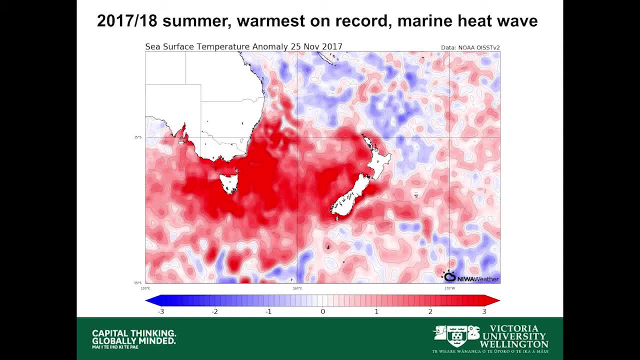 mean it was lovely in Wellington, really enjoyable, but I'm not so good for glaciers and you can see here. one of the effects of this is particular kind of climate setting we had over the. the summer was to have much warmer than average sea surface temperatures that stretch in a band all the way from. 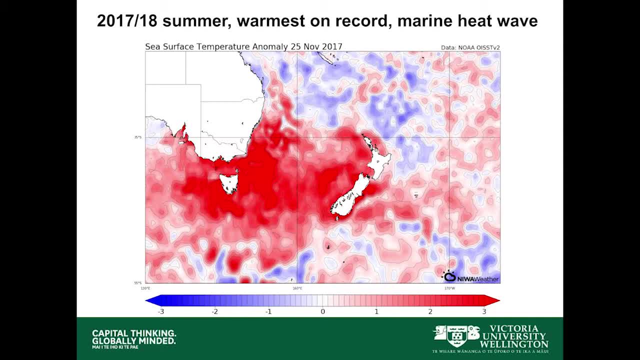 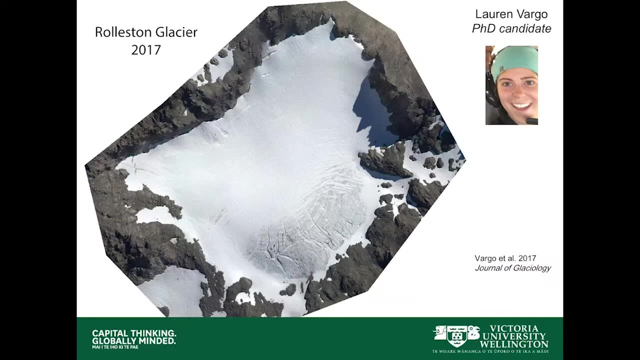 southern Australia, where I grew up, across to the cross to New Zealand. in the summer, And we've seen this historically. whenever there's a much warmer ocean around New Zealand, we tend to have terrible years for glaciers and if they occur in a sequence then we end up seeing ice retreat Lauren's here. 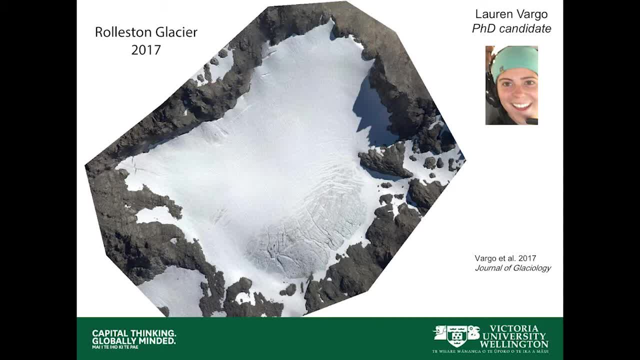 somewhere too, and she's currently working on using the photos that I showed you, a picture from inside the aircraft just before, but this is a photo of a small glacier, Rolston. it's near um. it's near Arthur's Pass, if anyone's driven over there. 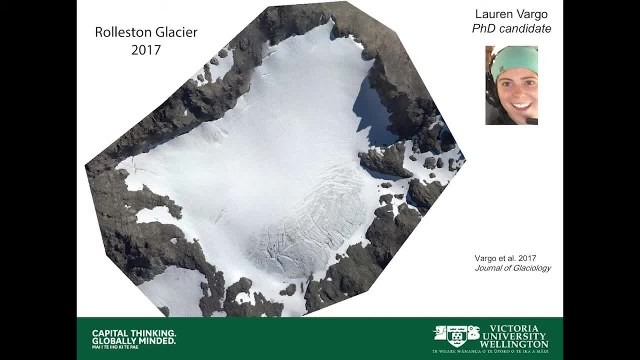 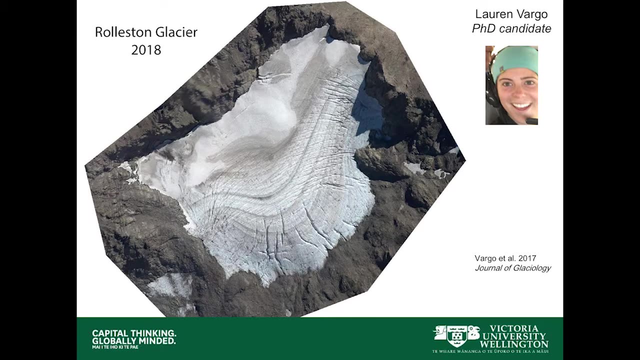 And looked up and seen the snowy mountains and this is what a happy glacier looks like. you can see. it's mostly covered in snow at the end of the summer and this is before the big warm summer. it's actually the, the big. it's the sort of the beginning of that period, but by 2018, after the sort of 2017-18. 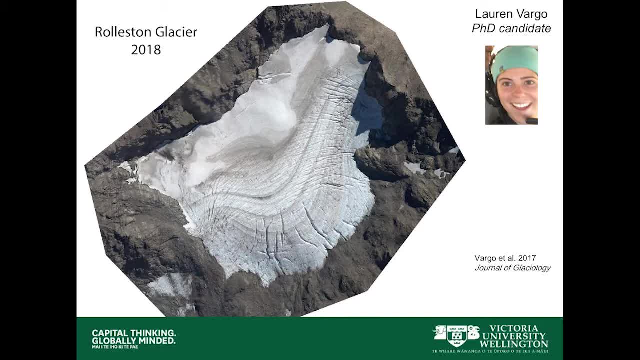 summer you can see what happens to a glacier when you have such extraordinary sort of raised temperatures and and warmer sea surface temperatures, or around New Zealand, right. so if these sorts of conditions continue, it's glaciers are going to be history. So on that note again, here's some work that. 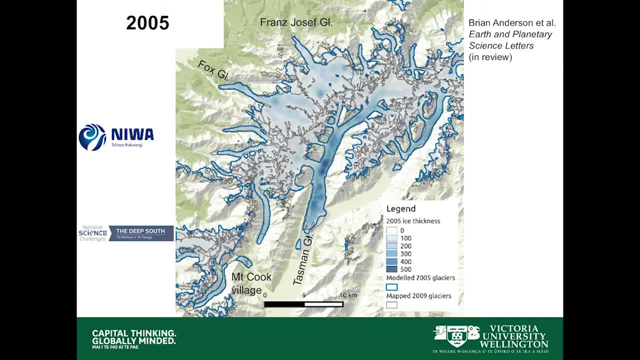 some that Brian and I are working on together at the moment looking at future simulations for glaciers. This is a sort of a close-up of the central part of the Southern Alps around Araki, Mount Cook. so this is Mount Cook village. for those of you who have been there- Tasman glacier, Hookah glacier terminus- you can walk up this valley. it's very interesting. 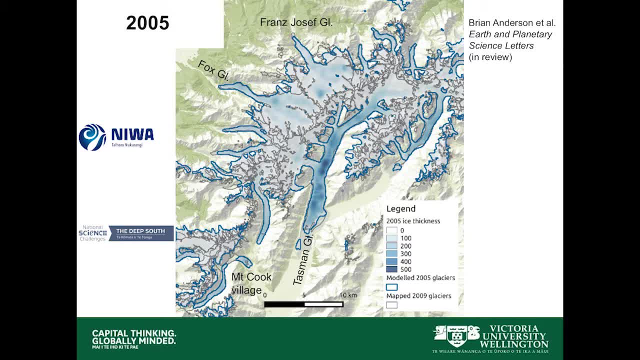 Nice Fox glacier and Franz Josef on the west coast right. so this is a part of New Zealand that contains about two-thirds of the ice volume and it's sort of representative of what's going on elsewhere, and it's a simulation with a glacier model incorporating all of the evidence that we've been collecting over. 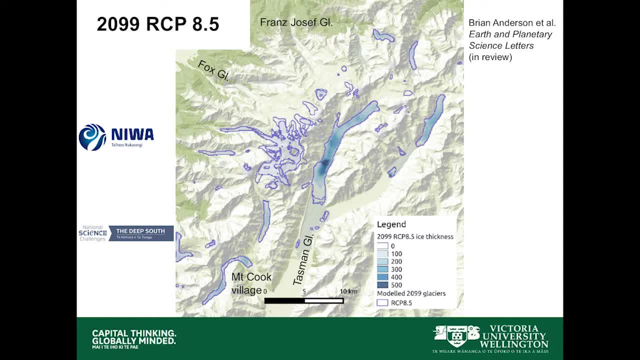 the years and in a simulation looking forward in 2099 under what's called RCP 8.5.. Now, RCP 8.5. I don't even. I don't even think I want, I'm not motivated to do that. I don't even. I don't even think I want, I'm not motivated. 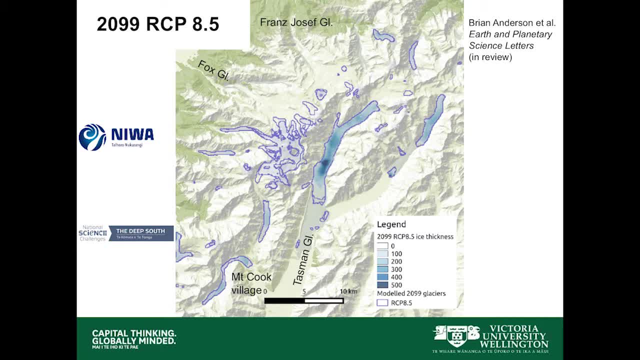 to explain the acronym. what I would say is: this is a climate where there's been no attempt at mitigation, so we sort of burn it all right and stuff the consequences. that's. that's more or less what RCP 8.5 is all about, and you can 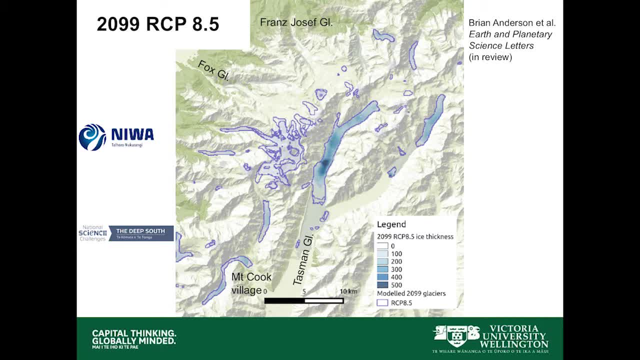 see that the consequences for glaciers are severe. in fact, they're mostly gone and we're left with a little bit of ice sticking around the highest peaks, and this is debris covered ice in the valleys. and if we play around with different types of ways of treating this mathematically, 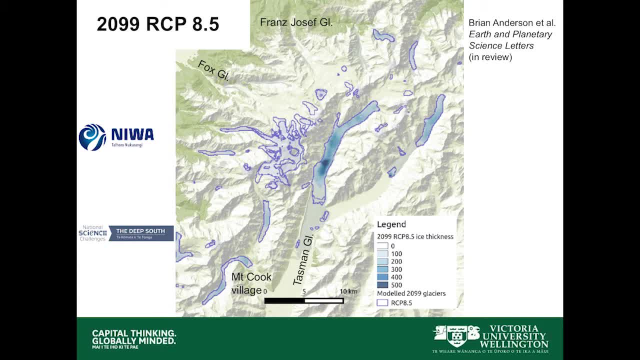 sometimes it goes and sometimes it stays, so we're not really certain about that particular result yet, but I think that the the message is clear. right, if you have unmitigated climate change, then glaciers are going to disappear, and this is true globally as well. right? so these are new, refined estimates for New 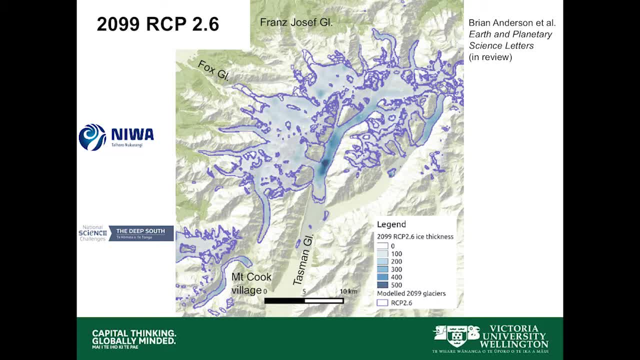 Zealand, but we see other similar things elsewhere, but under RCP 2.6. and this is a world where very intensive climate change mitigation has been carried out. in fact, we're drawing carbon out of the atmosphere, we've taken our budget down to zero and we limit warming of the atmosphere to around two. 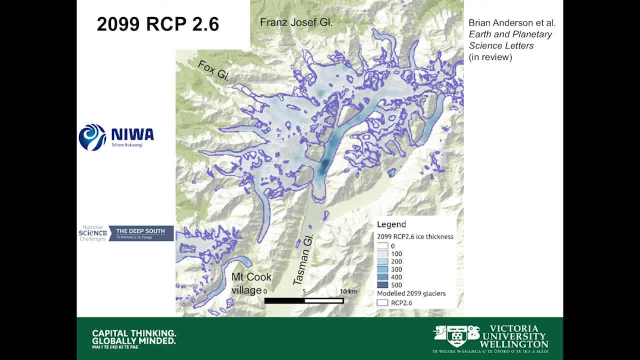 degrees above pre-industrial temperature. so in essence, this is the Paris agreement. it's not exactly, but it's close enough. you can see that glaciers remain. they're smaller than today, but they're still recognizable elements of the mountain system. under this sort of situation, they're still the that you 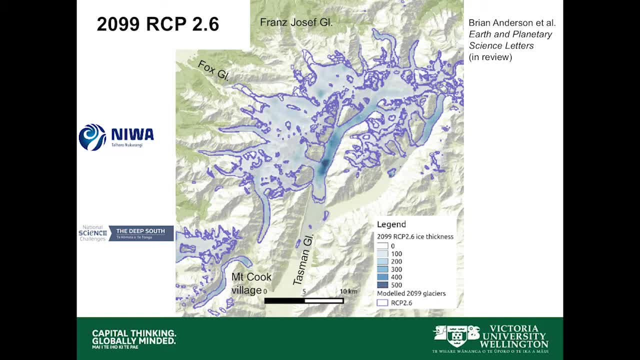 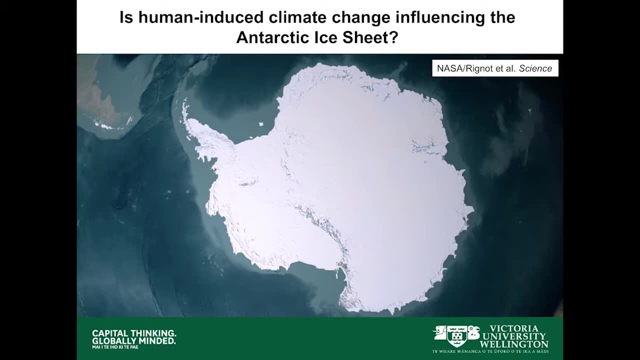 know the icons of the Southern Alps. we haven't lost them entirely. you know a people's grandchildren and so on would still get to see glaciers under this sort of scenario. so our choices in terms of climate change matter. I'm going to switch to Antarctica, right? so rather than just dealing with little glaciers, 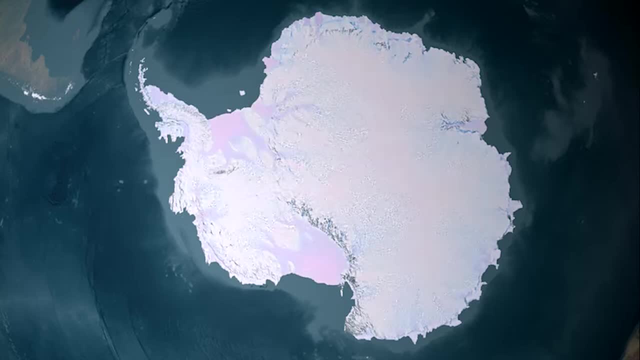 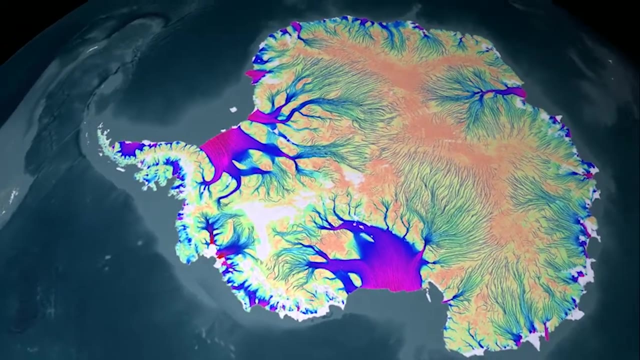 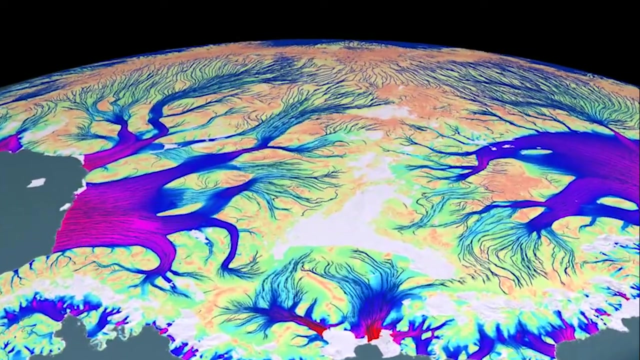 now we're talking about an ice sheet. in fact it's a number of different ice sheets. it's like a giant glacier. it flows from the interior out towards the coast. the colors here represent ice velocity, so where the dark, blues and purples are, the ice is flowing fastest. this is the most rapidly changing part of Antarctica. just 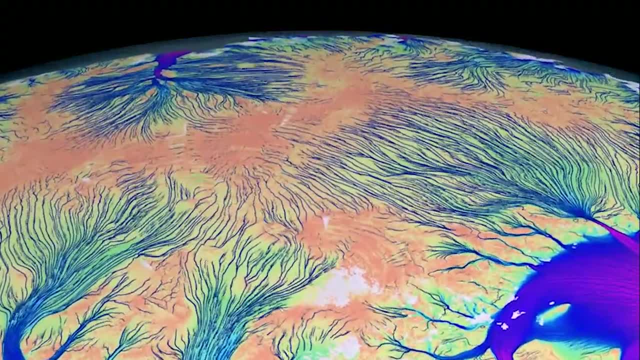 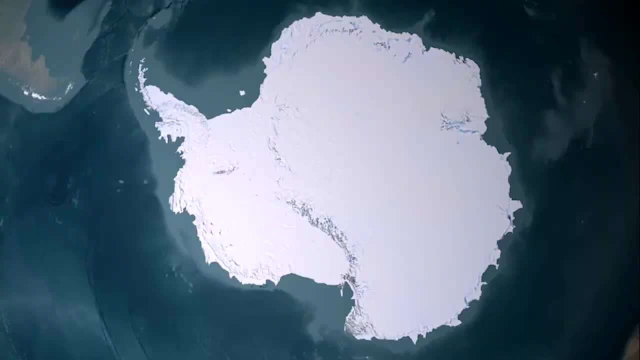 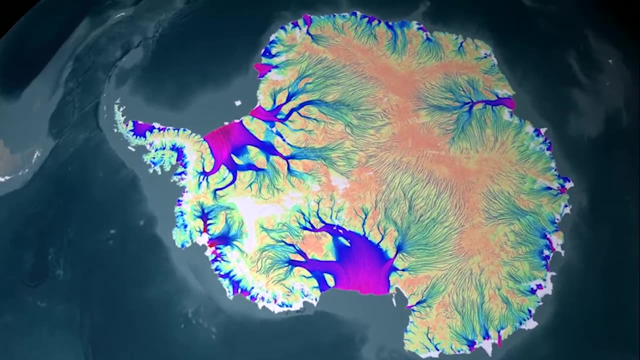 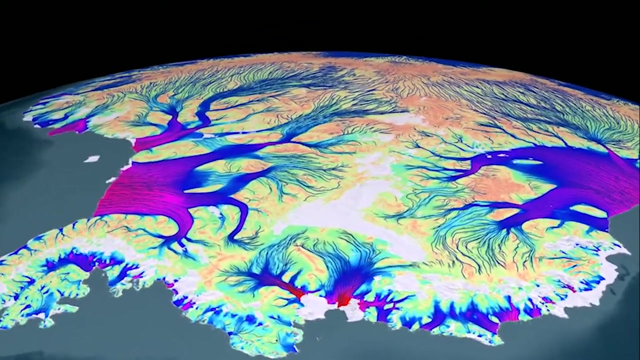 disappeared. it flows from this large, slow flowing part in the center. this is where people take ice cores to get sort of climate history. now one more time, because so much of the massive Antarctica is is lost through these fast-flowing ice streams. I think they're the key to understanding what Antarctica is going to. 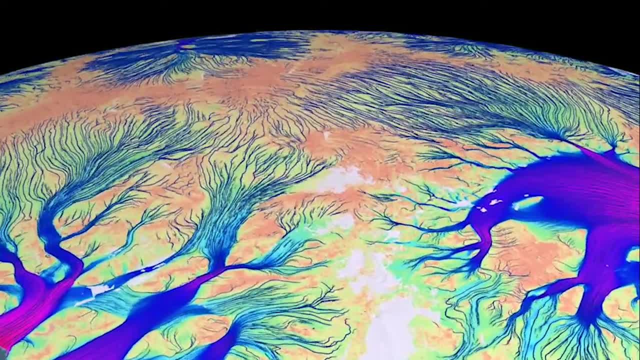 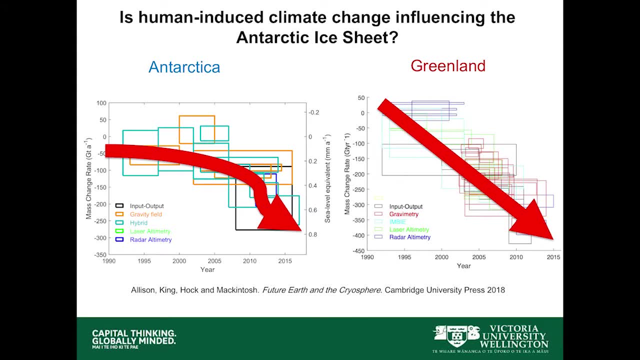 do in the future is to really understand the behavior of ice streams. so these two in particular, just we're just flying over them really in trouble at the moment. so this is another science plot. I'm going to explain it to you. it shows what's been happening to Antarctica and Greenland over the last few decades. 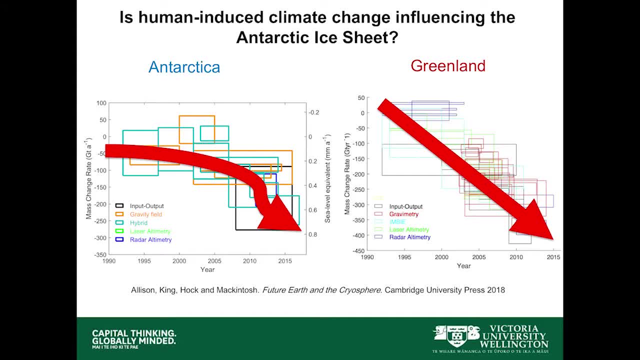 there are a few things to say. first of all, since 1990- that's really just about when we started to make the first quantitative observations of ice sheets using satellites, so we've only got a few decades of history of ice sheets. ice sheets actually take thousands of years to respond to climate change, so that's a 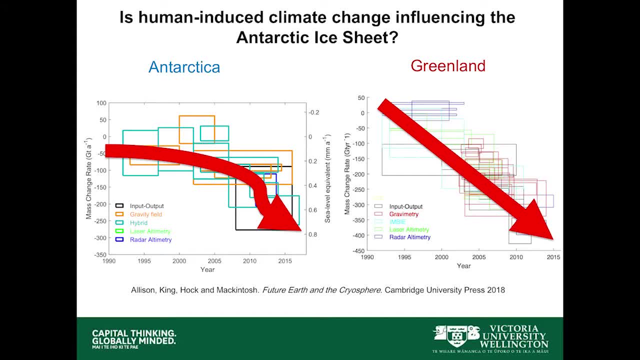 problem, right these boxes. each one of them represents a particular period of study and the y-axis represents the uncertainty of the of the estimate. so you can see uncertainty here and period. for Greenland what we've seen is, since 1990, a pretty uniform reduction in in ice mass loss. I mean there's been sort. 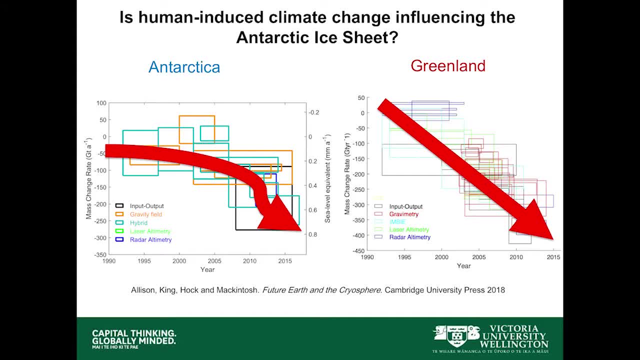 of continuous ice mass loss. right now that's contributing about a millimeter to sea level rise every year, so it's overtaken glaciers as the biggest contributor in Antarctica. the record is not so straightforward right. it started off being fairly neutral and there seems to be a lot of uncertainty in the 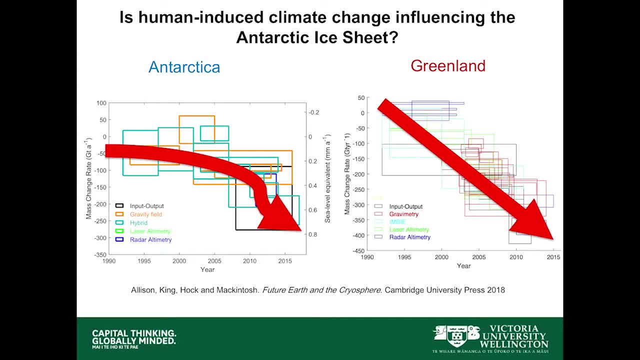 climate change in the mid 2000s. there's a new paper out that suggests that it was around 2007, the steepening and perhaps even a sort of sort of unsteepening towards the end. but Antarctica at least has the potential, we think, to contribute in a nonlinear way. in other words, you can force it, sort of. 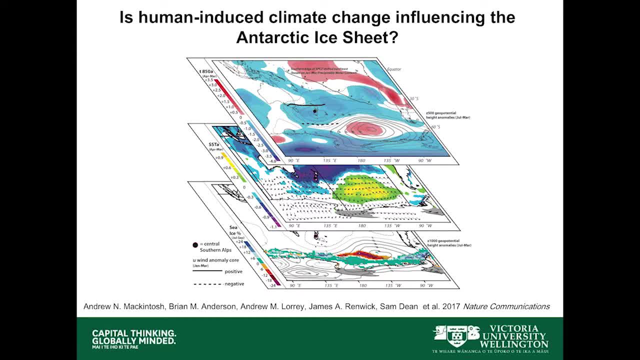 with, you know, the same climate and it will have a sort of larger response now. a minute ago I talked about New Zealand glaciers and the reason I talked about that particular paper is because it's a very interesting paper. and it's a very interesting paper is it has this interesting Antarctic element to it, as 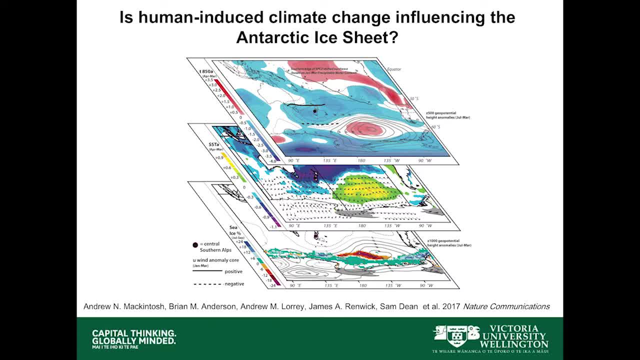 well. so the climate conditions that caused New Zealand glaciers to advance also caused a very large body of warm water to be located off Antarctica and stronger than normal westerly winds just off the coast, and those warm waters have been getting underneath Antarctic ice shelves and melting them. so this change. 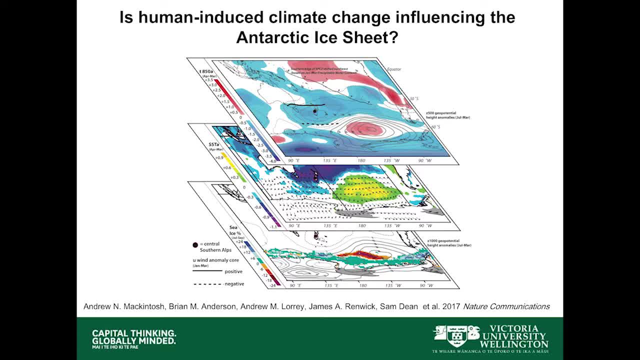 that I am pointing out here- it's actually a consequence of this, this one here as well. so, in other words, New Zealand glaciers can advance and you know, the West Antarctic ice shelf and the Atlantic ice shelf can finish off the straight and as it does that, that's a big one. and, to be clear, this curve out here: 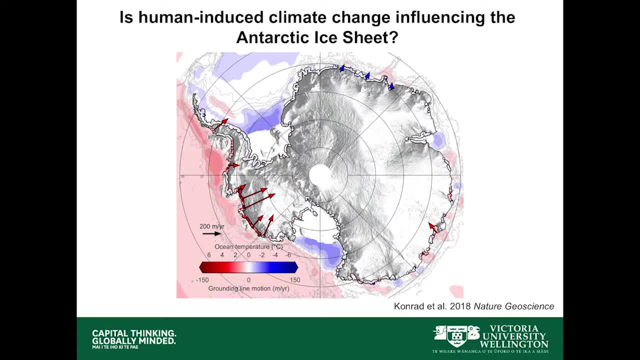 ice sheet can be destabilized by the same climate phenomenon and you can see this better here. so it's map showing west antarctica here, east antarctica, over here east antarctica hasn't been changing too much, a few sort of warning signs. things are going on over here at the moment, but 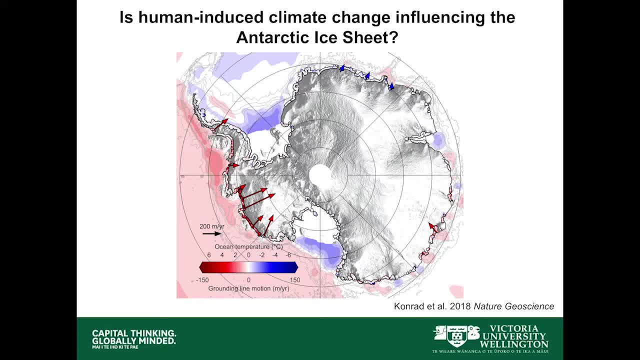 the major change in antarctica has been along the unincency embayment here and uh. this is where the arrows represent something called grounding line retreat, where the glaciers are starting to retreat from where they intersect with the, where the sea and the sort of ice peels off right that. 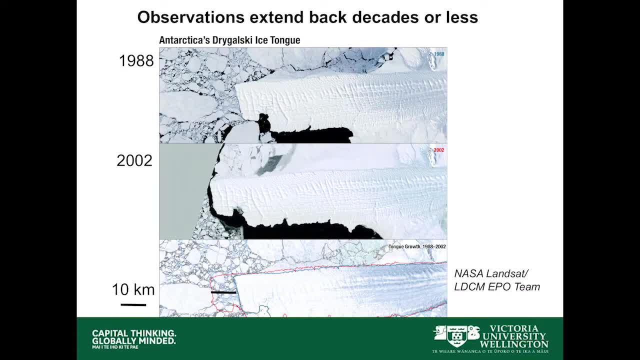 that line is starting to go backwards and, uh, this is just again to point out that, uh, we only have a few, uh decades of observations of of glaciers and in antarctica. so we need, we need to do better than that in order to understand a physical system that, um, that has this very long time scale. 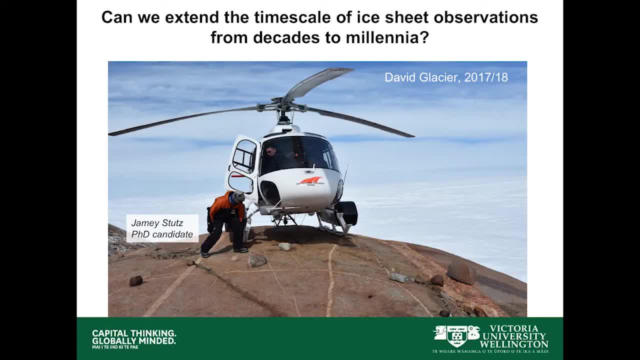 and, by the way, the dragowski ice tongue was the, the title slide of um of this talk, right? so how can we extend the observations if we, if we need to understand antarctica better? we need a few different things. we need a longer record of observations. 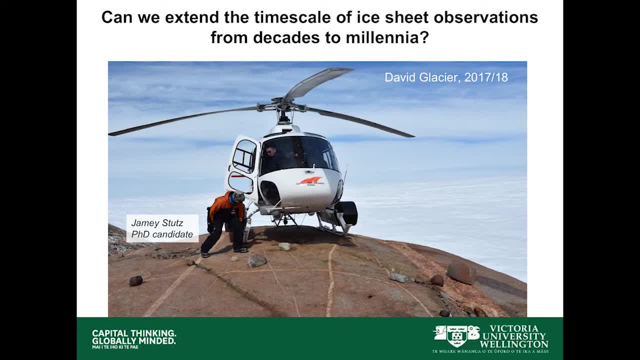 and we need better models of what the ice sheets are doing today. so one of the things i've been motivated to do is try to understand the history of the ice sheet over longer periods, and this involves doing field work in antarctica, so you can see here a squirrel helicopter for 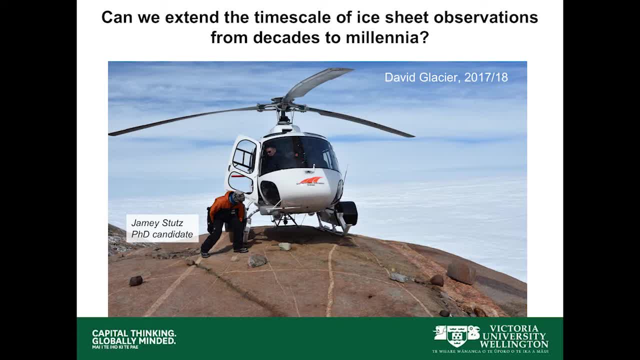 example, but you know i'm not quite interested in helicopters. um, yeah, and that the squirrel has almost landed directly on the sample that we're trying to take, which is just in here, and that's jamie, phd student working on this project, sort of trying to get under the helicopter. 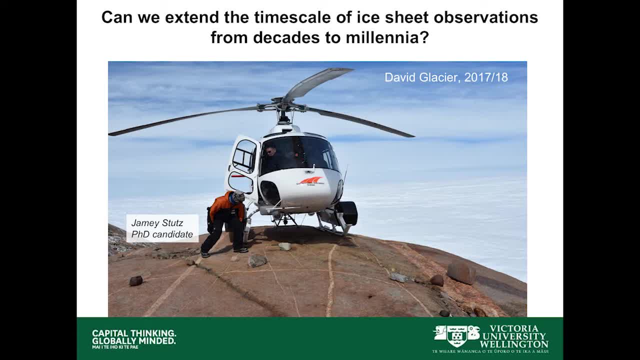 and pick up that rock before it gets knocked away by the helicopter pilot. so, anyway, there's a bit of a hint here that collecting rocks can tell us about ice sheet history, and you can see a big outlet glacier beside us here. this is david glacier, which, by the way, drains an area about the size of 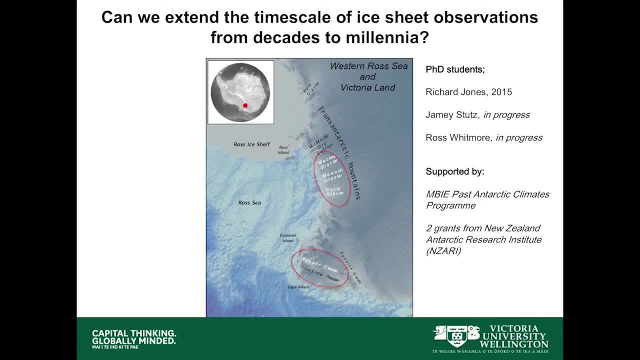 It's a huge glacier, And here's the coast of Antarctica and the Ross Embayment. New Zealand has a base just here- Scott Base- and we've been working on a bunch of outlet glaciers along this coastline. This has involved three PhD students so far, NB project and so on. right to really understand. 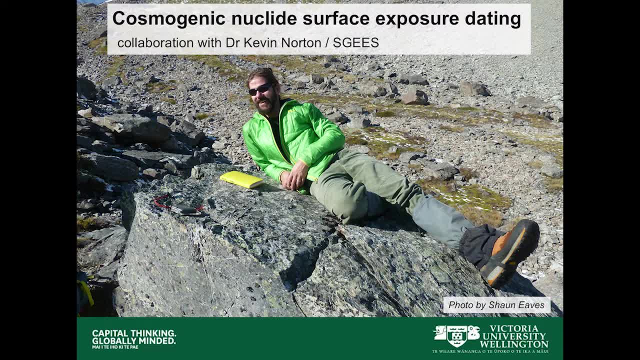 the long-term history of the ice sheet. Now this work's sort of been made possible through collaboration with Kevin Norton, who we appointed in SG's as a lecturer a few years back Now. Kevin's an expert in using cosmogenic isotopes to understand Earth system sort of. 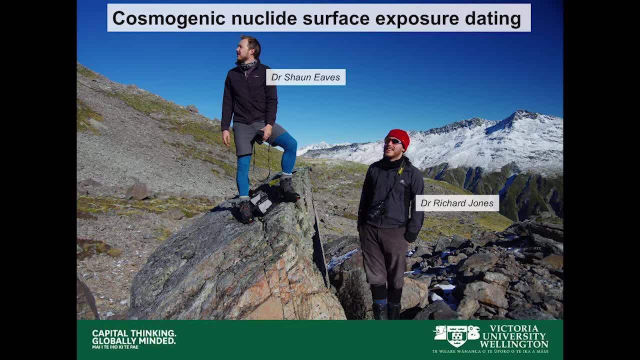 processes, And a few years ago, Kevin and I appointed two PhD students, Sean Eaves and Richard Jones, to work on this particular problem, to try to sort of reconstruct glacier and ice sheet history using cosmogenic isotopes. It's been fantastic. 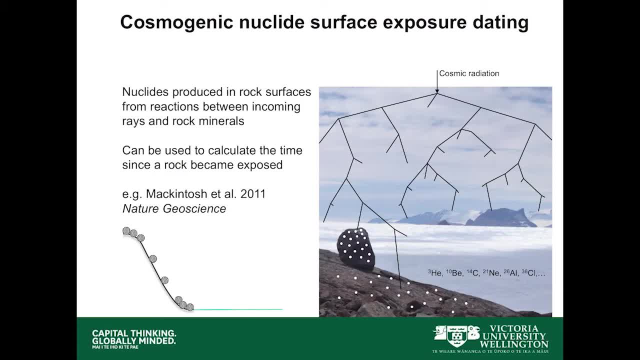 So I'll show you what this is all about. You can see a glacier there in the background, a big rock in the sky, And every day we're bombarded by cosmic rays. They come from deep space. Mostly, they're created in supernovae. 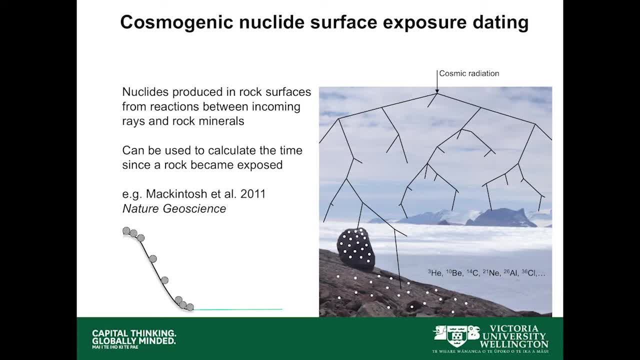 And they make their way down to the surface and cause small changes in the chemistry of rocks that sit at the surface. So you can see the rock there with a pile of little white dots on it where cosmogenic nucleides have been accumulating through time. 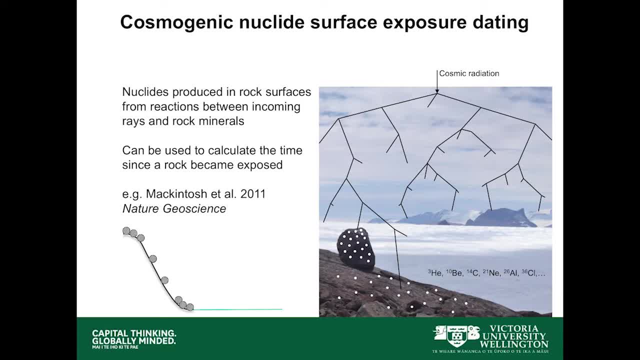 Now, if you take a look at the ice sheet, you can see that there's a huge amount of ice here. And if you take a glacier and look at a transect- a mountainside that's just abutted against the glacier- and collect rocks along that mountain slope, you can take samples and measure. 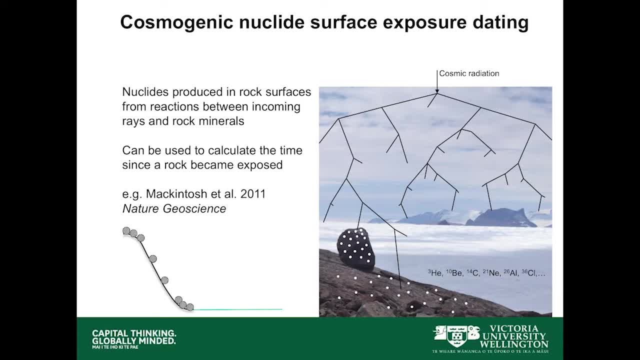 the cosmogenic nucleides inside them and reconstruct the history of that glacier. So you can imagine a retreating glacier. It will have a larger abundance of these nucleides at the top and fewer as you head down. Now This is a tremendously powerful technique for reconstructing glaciers and how they've 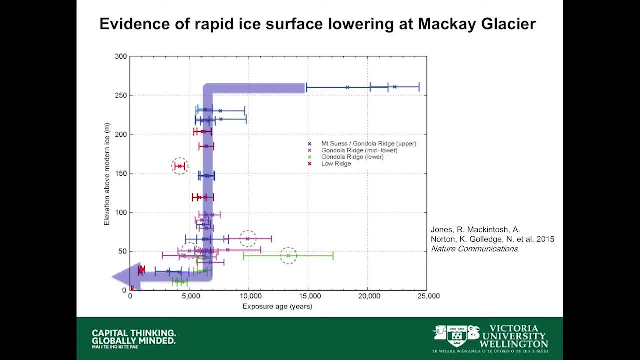 changed through time, And this is what one of the data sets looks like, And you know most scientists. you put a graph and a bunch of points. it doesn't look terribly exciting, right? But this one really is. On the y-axis, you can see the thickness of the glacier. 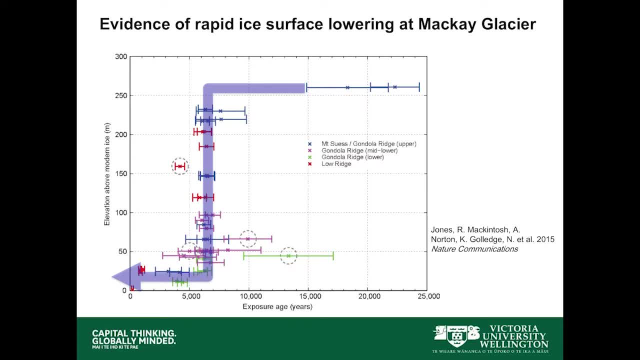 Sorry, the thickness of a former glacier up against a bedrock sort of ridge. And here is time, And each one of these dots represents one of a single rock that we've picked up from. you know, beside the helicopter. You know we actually have to walk uphill sometimes. 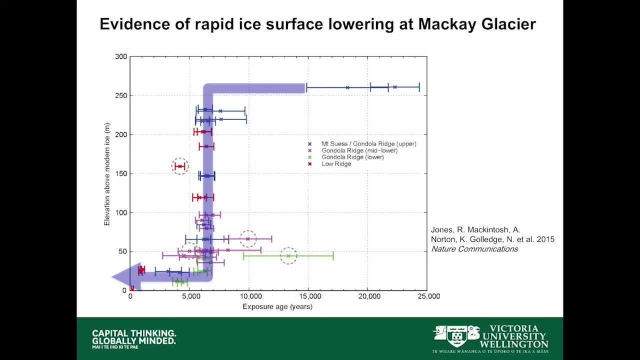 And so what this represents is a glacier that was 250 meters thicker than present sort of 10,000, 15,000 years ago, And then about 6,000 years ago, it underwent a rapid, dramatic thinning event: hundreds. 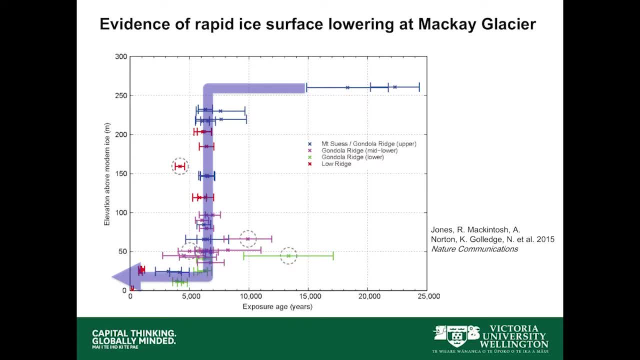 of meters, and in almost instantaneous time, In fact. we did some careful statistics on this and what we found was that this event probably lasted about sort of 500 years, And it involved thinning of the glacier at about the rate that what we're measuring. 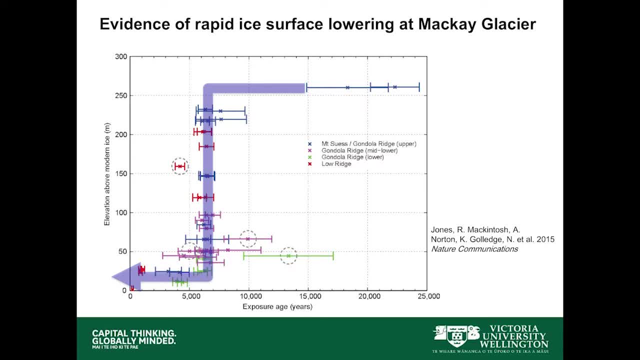 on the most rapidly changing parts of Antarctica today, right? So in other words, some of the thinning events that we see in Antarctica today have some precedence in, you know, the recent past. So there's some real value in extending the record of observations from glaciers sort. 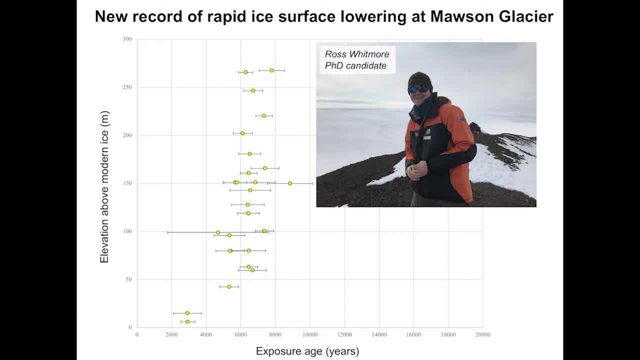 of back through time. You kind of wonder, you know, when you get a result like this, is it just a fluke, and you know, is it repeatable? And so we've been trying this at a number of different glaciers over the last few years. 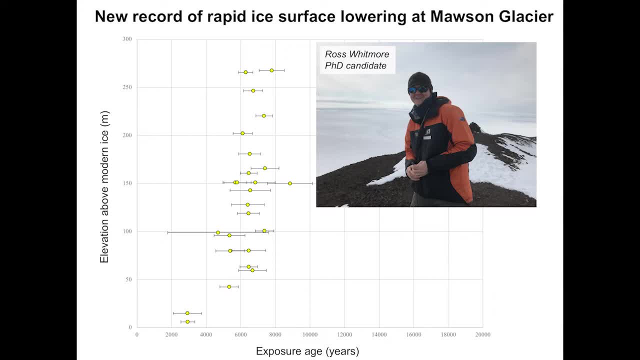 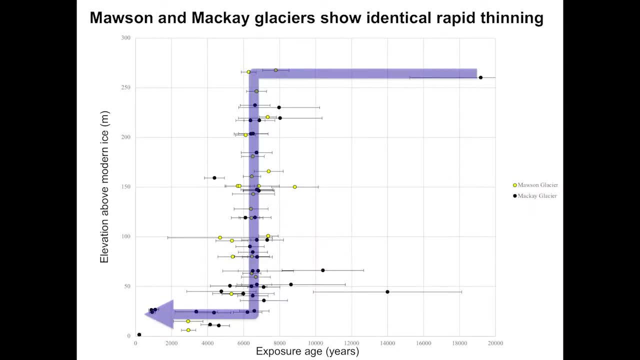 You can see a record- a new record here, from Ross Whitmore, another one of my students, and it's showing the same kind of behavior. In fact, if you put all of these ages on the previous plot and combine them, you end up. 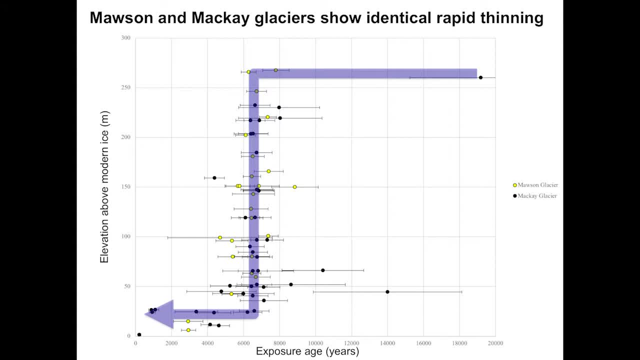 with another record that is basically indistinguishable showing the sort of rapid changes in glaciers in the recent geological past, And this was when we got this record back. we kind of scratched our heads a little bit right, because we weren't sure why something like this would. 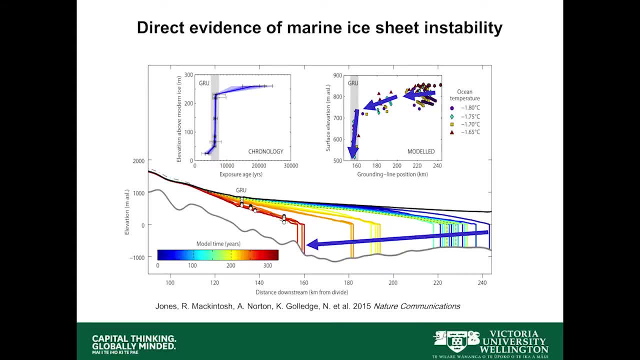 have happened at this particular time, And what we found is that. so again, my group's been sort of trying to date rocks and understand glacial history, but also use numerical models to reconstruct glaciers through time, And what you can see here is a cross section through a glacier. 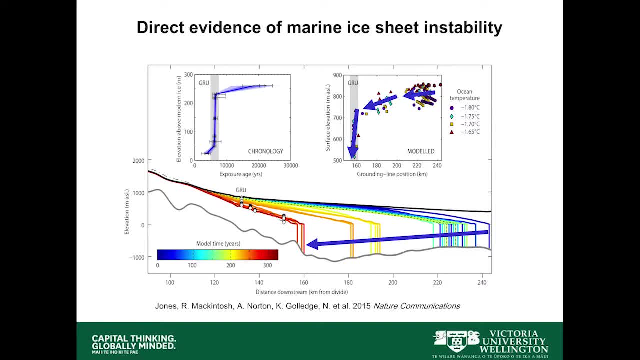 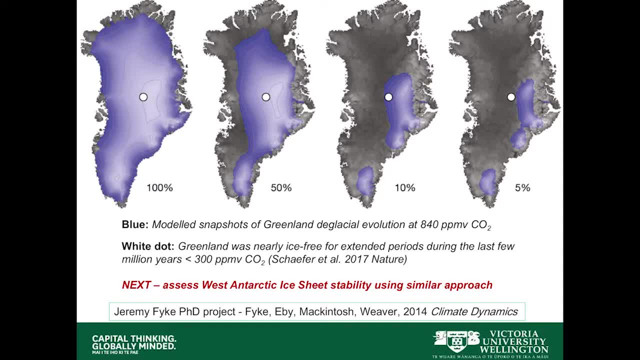 And here's the geological history of that glacier. And here's the geological history of that glacier. Um, but I'm switching to Greenland for a second. I had a PhD student a few years ago, Jeremy Fike. 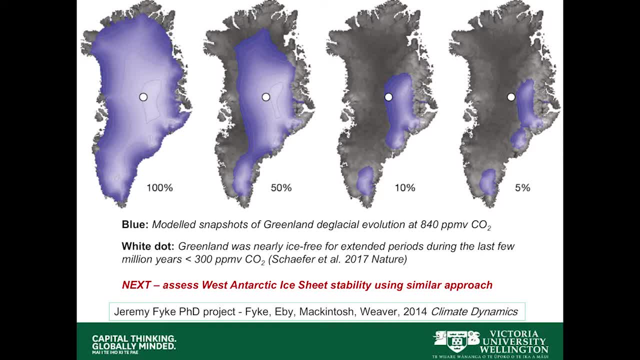 who looked the evolution of the Greenland ice sheet, how it was going to change over the next sort of few centuries to millennia, And he used a, a climate model that was coupled to an ice sheet model, so it included all the appropriate processes. 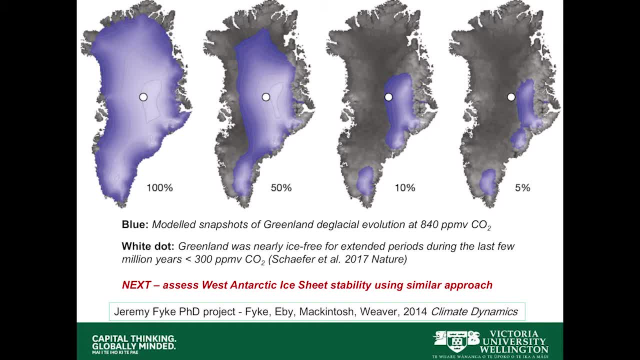 And you can see here a future simulation of the Greenland ice sheet under 840 ppm CO2.. This is approximately twice as much carbon dioxide as we have in the atmosphere at the moment And you can see that under an enormous amount of CO2,. 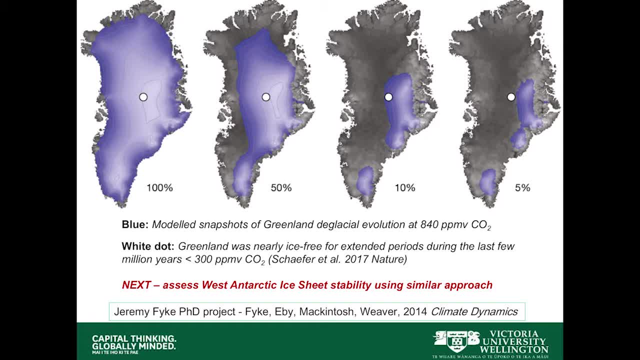 Greenland disappears. It takes a while. It takes thousands of years. It's much slower than Antarctica. It disappears in a certain pattern. However. recently, some of my colleagues took some samples of rock from this white spot in the center of Greenland. 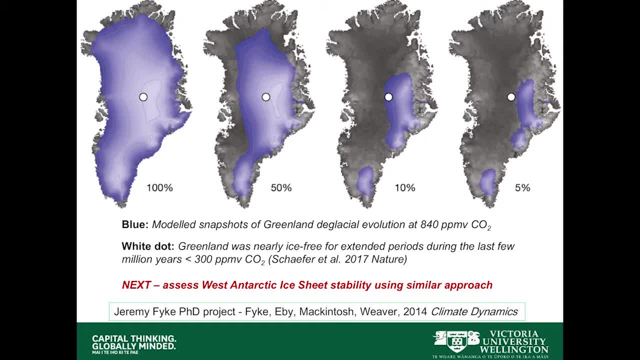 They used beryllium-10, this cosmogenic nuclei that I was talking about a minute ago, that Kevin Norton works on with me- And they found that Greenland had been nearly ice-free for a large part of the last few million years. Now we've had nothing like 840 ppm of CO2. 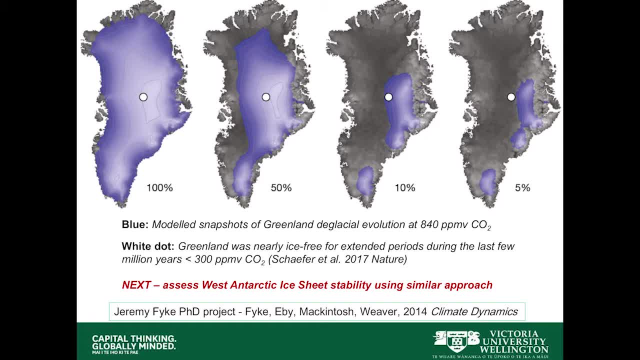 in the last few million years, It's only been a few hundred parts per million, somewhere between 200 and 300 at most. So So something's wrong here. There's either something wrong with this evidence that they made a mistake. I mean, I would love to see it replicated, to be honest. 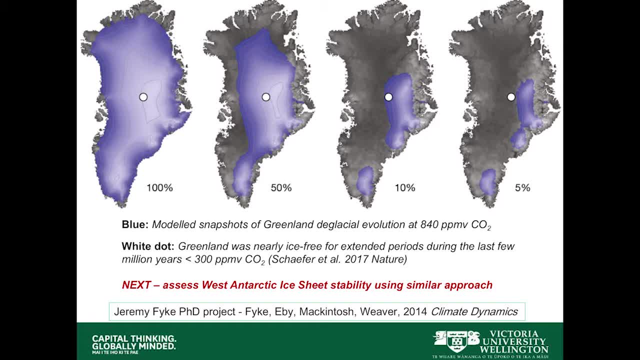 It'd be nice to see some more samples like this, But they come from the bottom of ice cores And it's very hardly one material. You've got to put a multi-million dollar project to drill to the bottom of an ice sheet and collect a little bit of sediment. 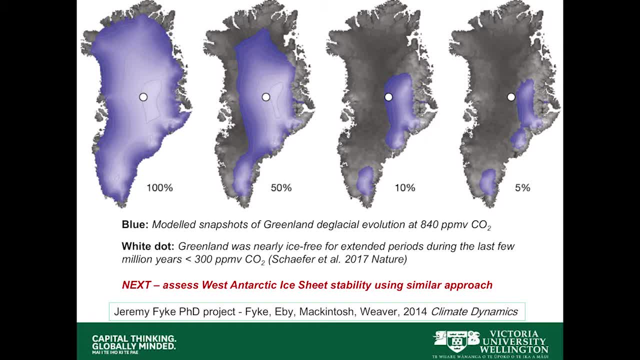 and then measure the beryllium in it. There's not much chance to replicate that, Or there's something wrong with the model, And I think that ice sheet models are getting pretty good these days. They're pretty good at simulating ice dynamics. 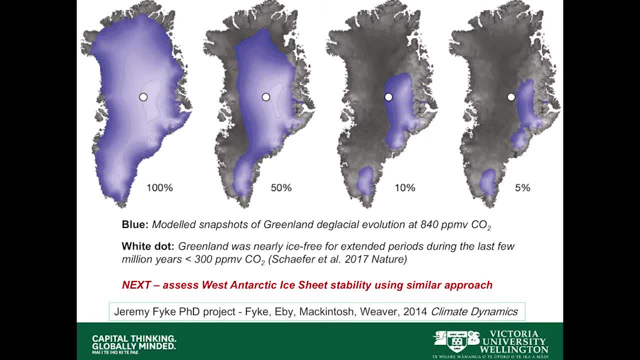 But the real problem we still have is the coupling between the climate system and the ice sheet, And there's a lot more work that needs to be done in that space in order to make what I think are realistic future projections of ice sheets. So if this doesn't work for Greenland, 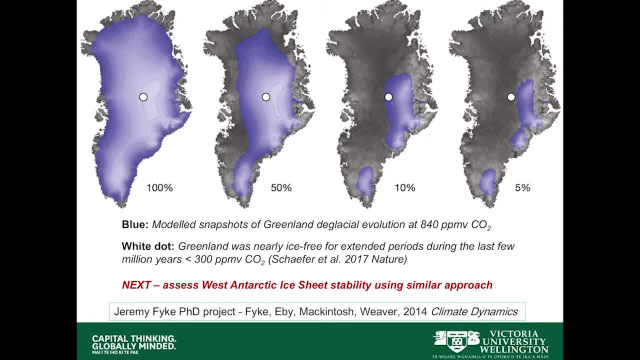 it's not going to work anywhere And we've got our sights on trying to do similar sorts of work in Antarctica, where we try to get sediment from beneath ice sheets to find out whether the ice has been missing in the past. I think we can do this in West Antarctica. 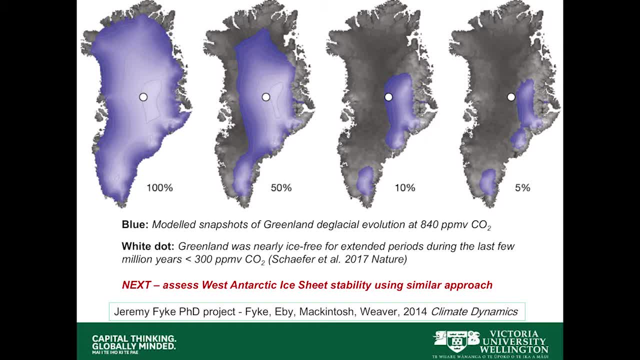 And then we'll combine that with our best possible numerical models of ice sheets and try to sort of test them out on that sort of past evidence, And then I think we'll have more confidence in future projections. It's only at that point when we'll be able to do it. 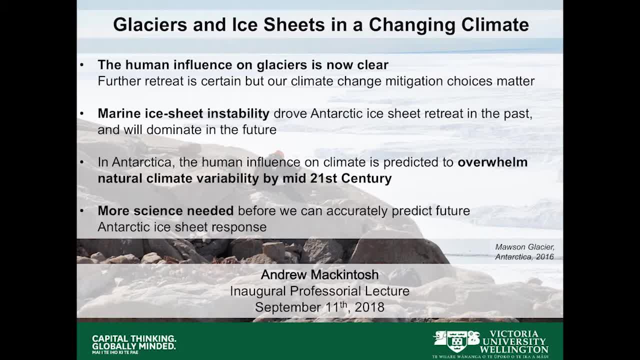 Right, So I could even be slightly early, but I think that's OK. I think the human influence on glaciers is now clear. Since about the 1990s, the influence of fossil fuel burning on the climate and then glaciers has become very, very clear. 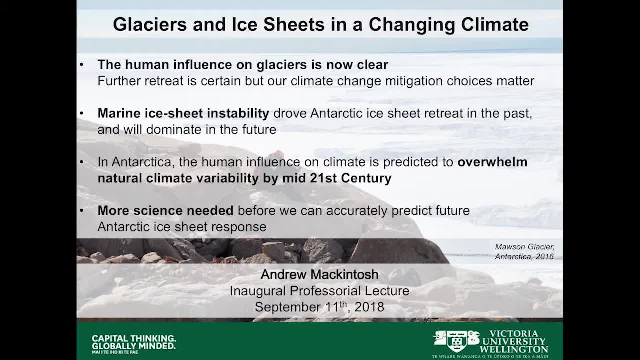 Of course, regional climate variability still causes glaciers to advance and retreat a little. We've seen an example of that in New Zealand. But further retreat is certain and our climate change mitigation strategies really matter here. So I gave you an example for New Zealand. 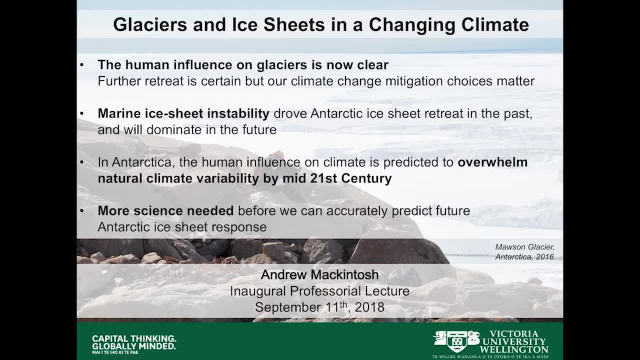 where you saw, under RCP 2.6, the Paris Agreement, we kept glaciers Under 8.5,. we lost nearly all of our glaciers. So what we do there as a society and as a planet really matters. And marine ice sheet instability, drove Antarctic ice sheet. 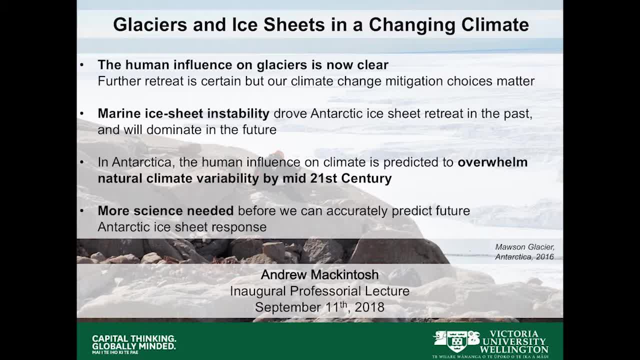 in the recent past and it's going to dominate in the future, in particular in those areas where we see warm water getting underneath ice shelves. That perhaps unstoppable process of marine ice sheet retreat is going to make a big difference in the next few centuries, with major impacts on sea level. 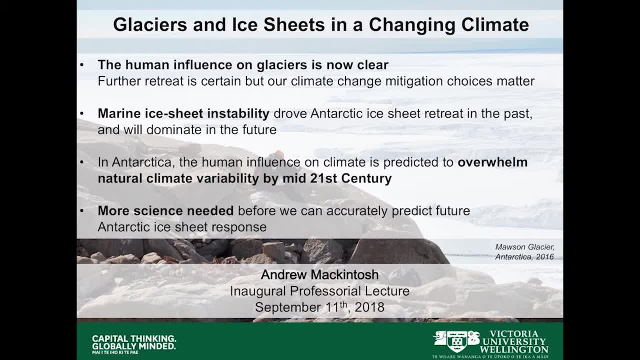 and climate change And really changing the face of our planet. And because Antarctica is currently pretty cold, there's quite a variable climate that's influenced by tropical processes. I mean that sort of multi-layer plot that I showed with the different parts of Antarctica. 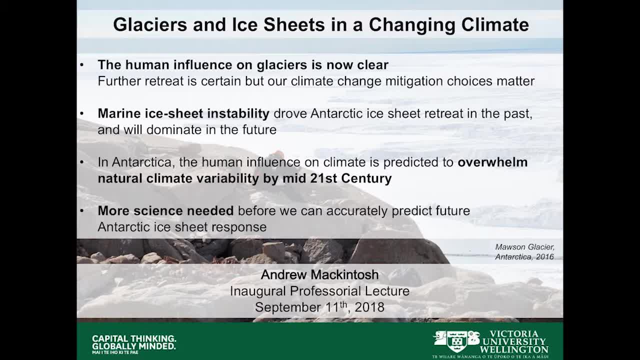 some were growing, some were getting smaller. That natural variability in the climate system is still very large. But climate models predict by about mid-21st century human processes are going to start to overwhelm That, just like they have for glaciers a few decades back. 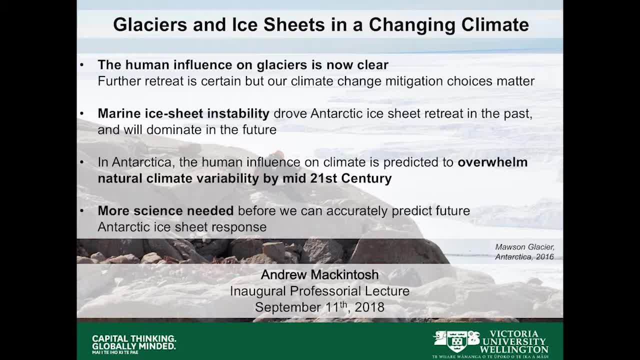 So I think that what's going to happen in the future of Antarctica is still looking pretty bleak, And again, our choices matter, but there's a lot more to do with the models. before I really believe what future simulations say, And so if there's a plug at all there, 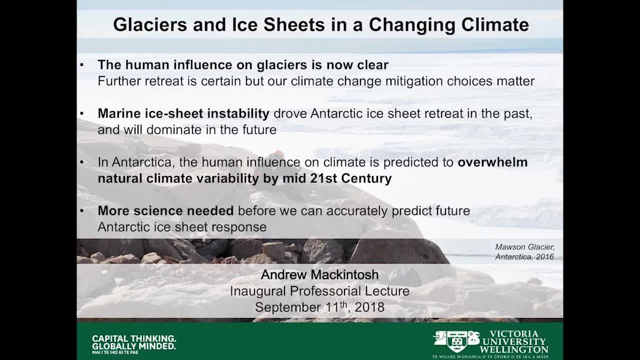 it's that we need more science in order to understand the system properly. This is not a solved problem. I mean, I was personally pretty disappointed a few years ago when in Australia There's a move in CSIRO to stop doing climate change science.